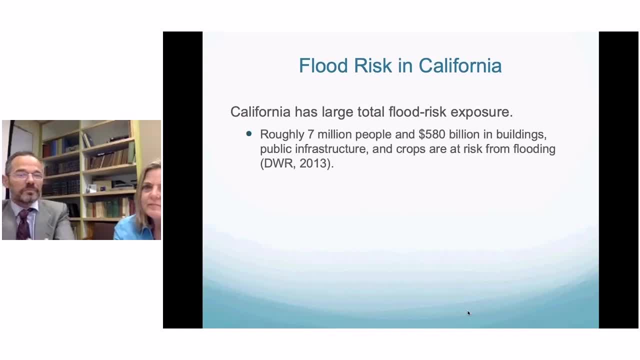 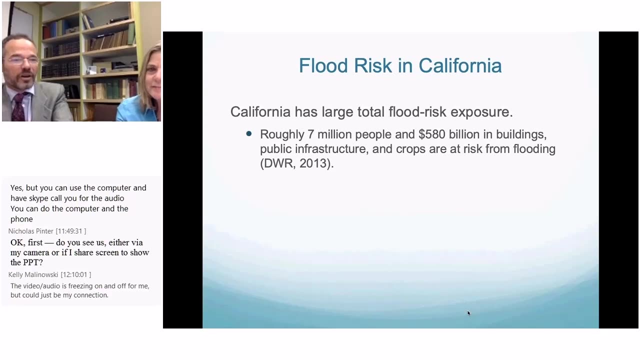 extensive total flood risk. It's been estimated that 7 million California residents and something like $580 billion in infrastructure and crops are at risk of flooding within the state, And my understanding is that is based on the 500, so-called 500-year flood zone. Other people have 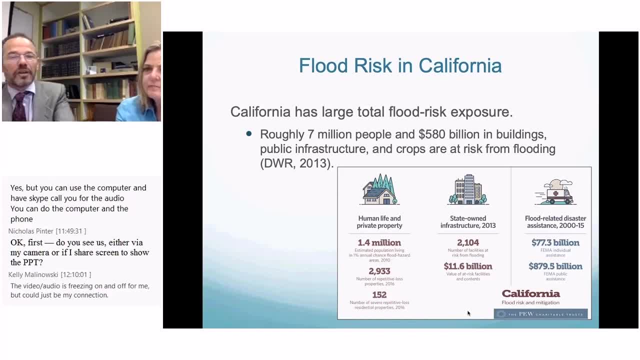 looked at this. For example, Pew Trusts did a study of this, focusing on the smaller 100-year flood zone, and came up with a study that showed that the state has an extensive total flood risk, And that's comparable numbers: millions of Californians and hundreds of billions of dollars of infrastructure at risk. 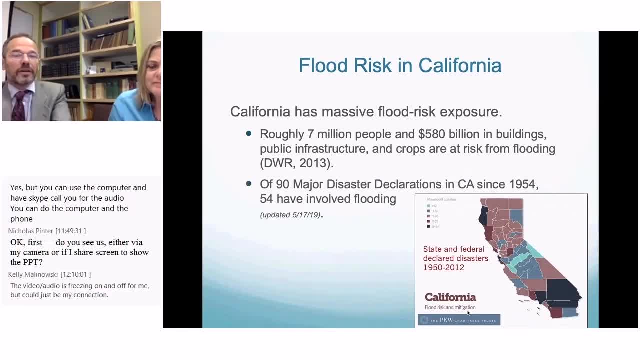 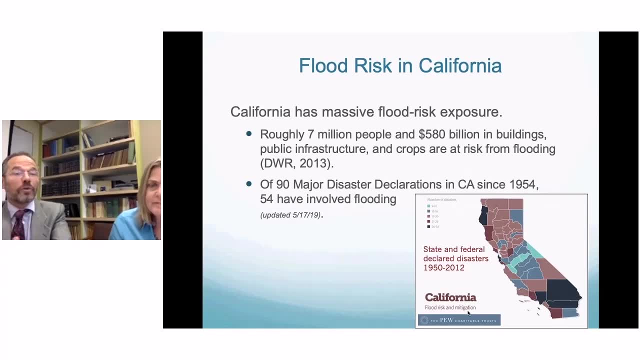 So, looking back historically, of 90 major disasters declared within the state since 1954, 54 of those- or 60%, exactly 60%- actually have been flood-related. So we've an extensive history of flooding And the major tool for. 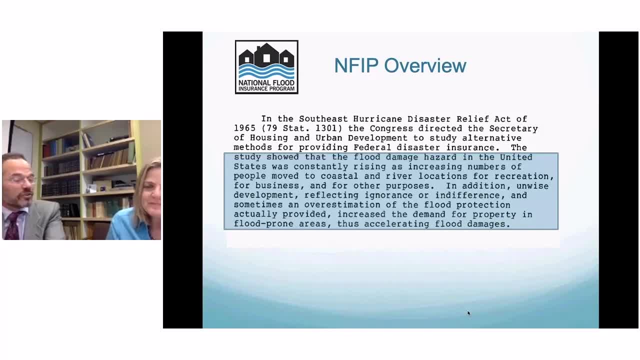 managing flood risk in the state and nation wide is NFIP, of which Kathy has some experience. So in 1965, Congress passed the Hurricane Disaster Relief Act And in doing so they asked HUD to study alternatives to the National Flood insurance program, or asked HUD to study 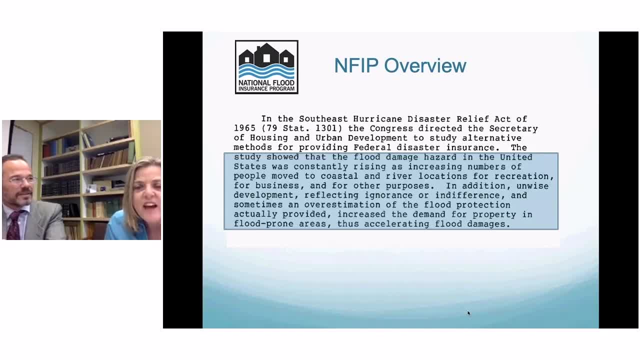 alternatives for a insurance program, And the report that came out found that, in addition, these measures change forecasts so that the nature of risk-玐 of vezes, when water dollar and new dollar is pushed under each other, conditions start to change for better insurance. But we don't have all the information in the US today about 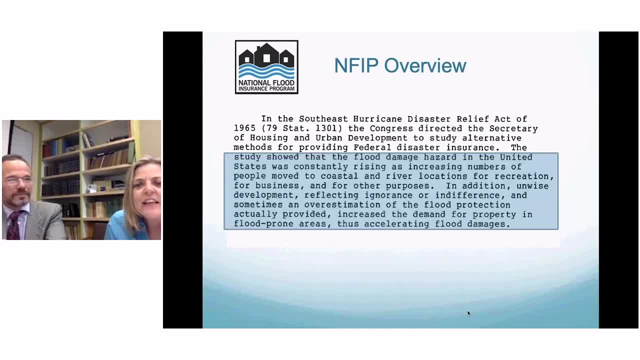 it exactly. The actual water dollar in Florida is that they're all leading waste management workerOh. In addition, unwise development reflecting ignorance or indifference and sometimes an overestimation of the flood protection actually provided increased the demand for property in flood-prone areas, thus accelerating flood damages. 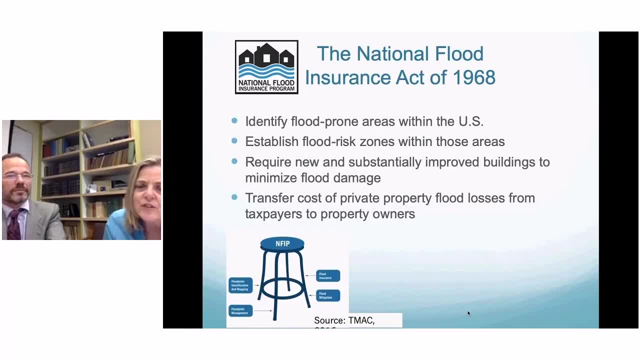 That report led to the enactment of the National Flood Insurance Program in 1968. And in 1968, the program was developed as part of a three-legged stool. It starts with a FEMA flood insurance rate map. The map is then adopted by communities and used to regulate development in the floodplain. 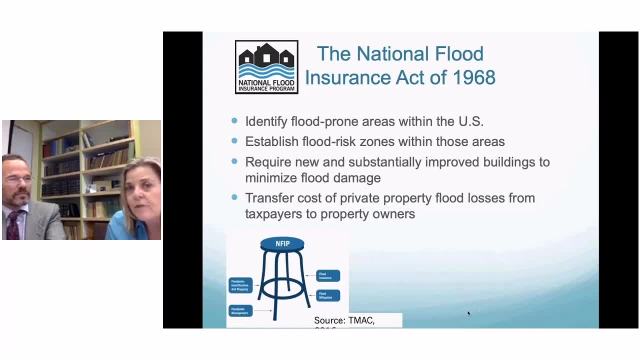 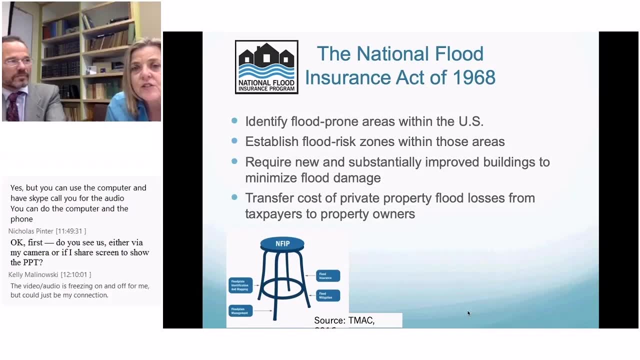 And then, in exchange, FEMA provides flood insurance to anyone and everyone who wants it. The time when the act was initiated, in 1968, it was initiated as a three-legged stool. With time, mitigation became the fourth leg of the stool, and so today it's considered a four-legged stool. 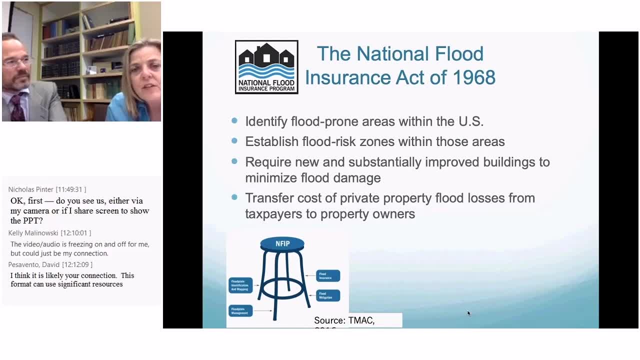 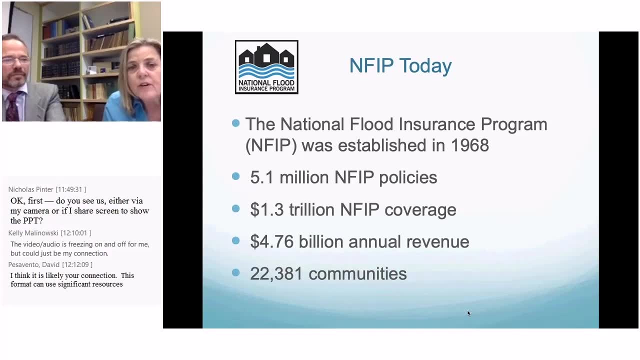 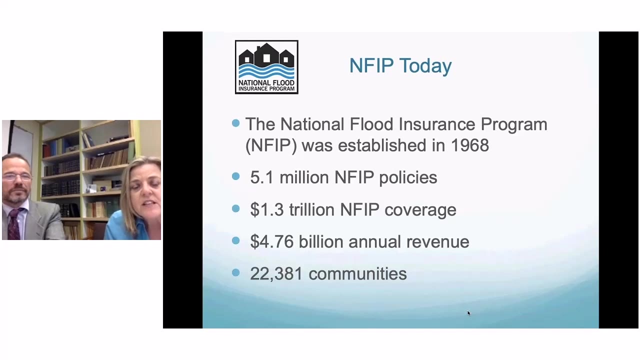 with mitigation flood maps, regulations and insurance. About a month earlier this month, Diane Horn from the Congressional Research Service gave a presentation to congressional staffers And in her presentation she gave the latest numbers for the NFIP. Today there are 51 million NFIP policies in force. 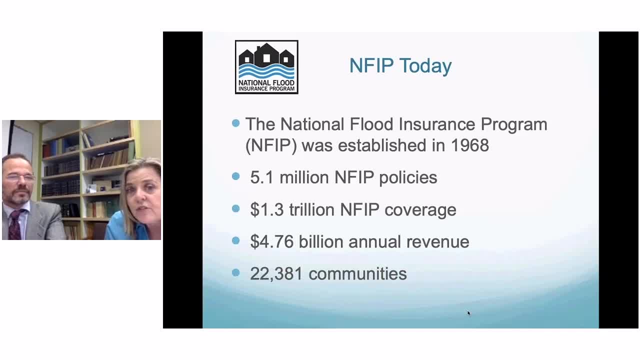 providing 1.5 million NFIP policies in force. providing 1.5 million NFIP policies in force. providing 1.5 million NFIP policies in force. providing 1.3 trillion dollars in coverage and 4.7 billion dollars in revenue. 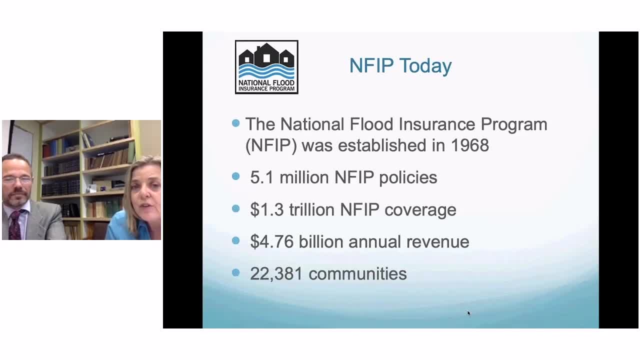 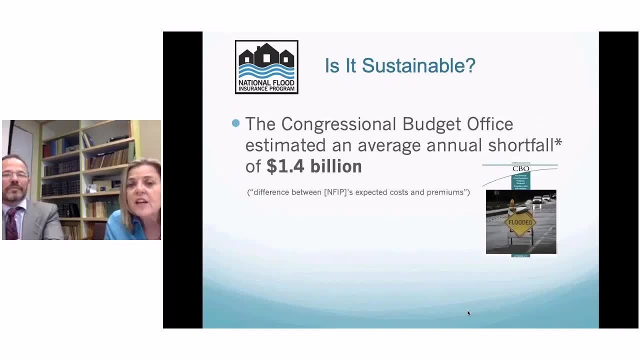 Almost every community in the United States is covered by an NFIP policy or has the opportunity to present an NFIP policy. That same or a similar report coming out of the Congressional Budget Office in 2017, estimated that the National Flood Insurance Program has an annual average annual shortfall. estimated that the National Flood Insurance Program has an annual average annual shortfall of 1.4 billion dollars. of 1.4 billion dollars of 1.4 billion dollars. That's the difference between what the costs and the expected premiums. 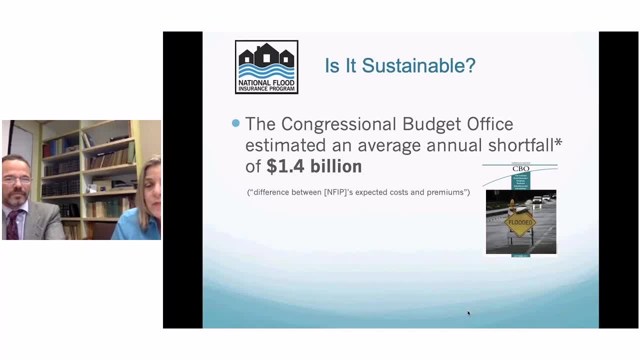 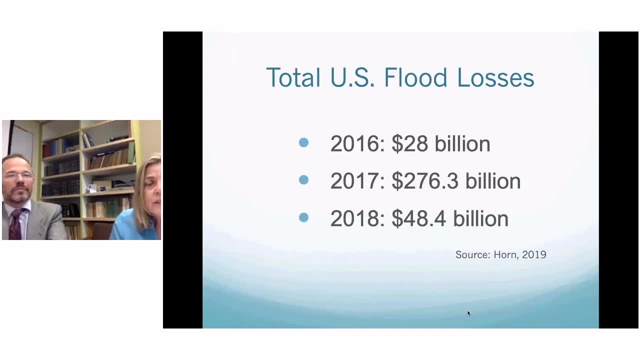 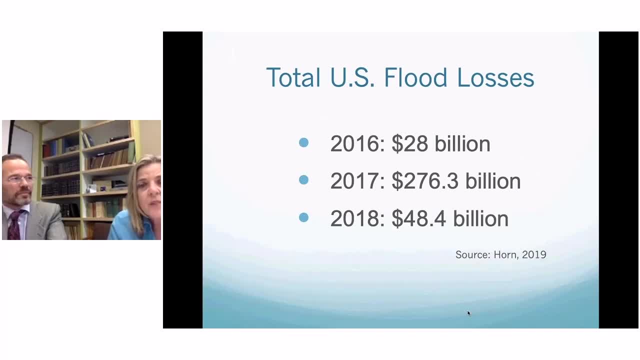 Diane also presented the current status of the flood losses. In 2016,, 2017, and 2018, the National Flood Insurance had major losses. Diane also presented the current status of the flood losses. Diane also presented the current status of the flood losses. 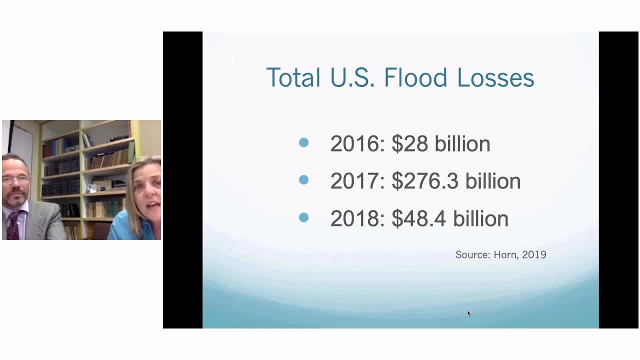 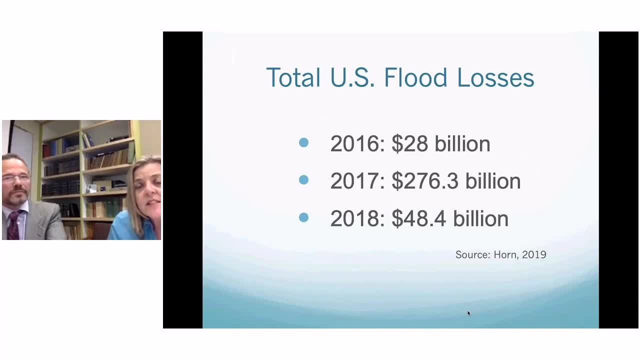 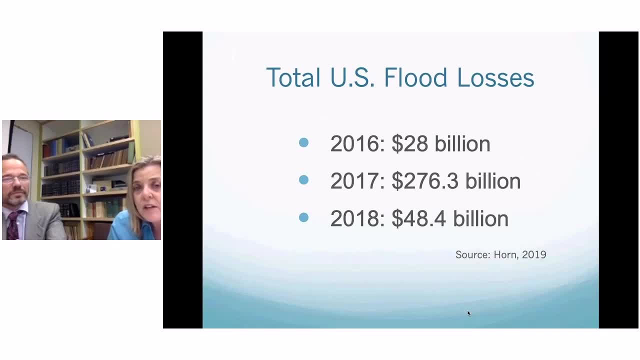 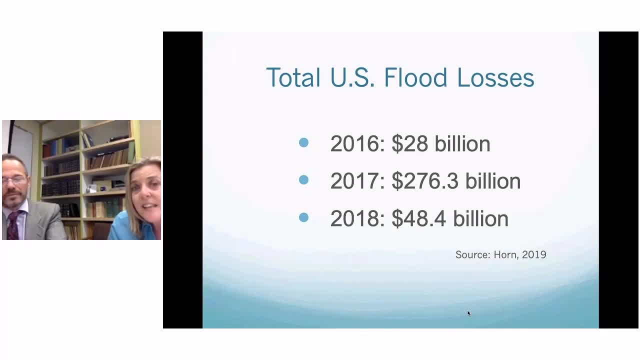 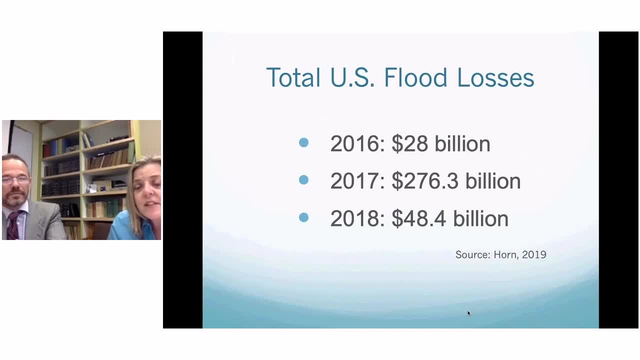 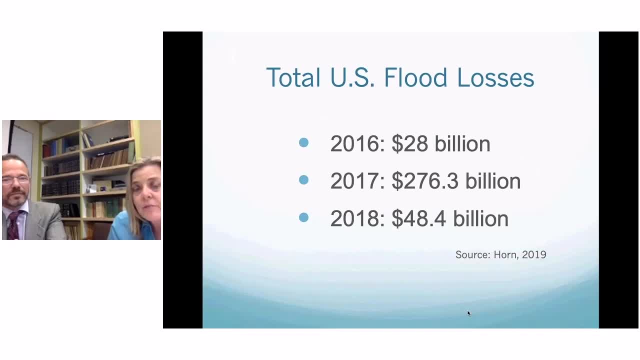 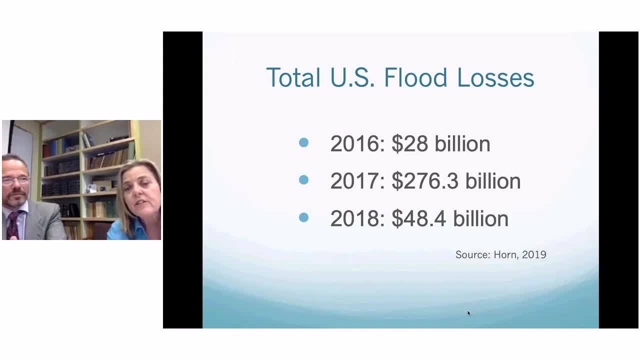 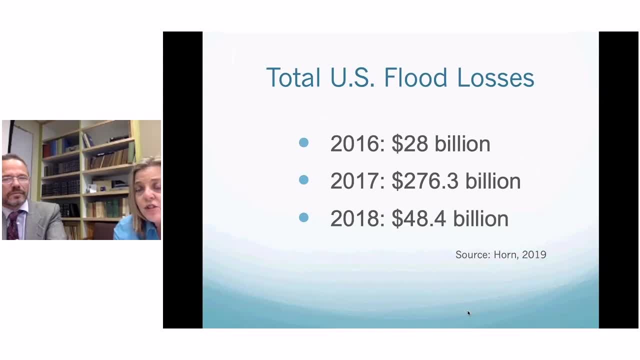 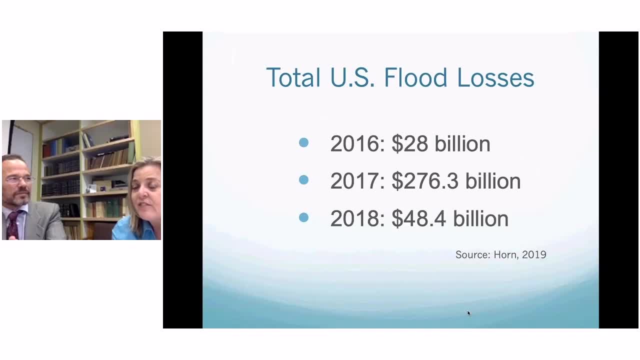 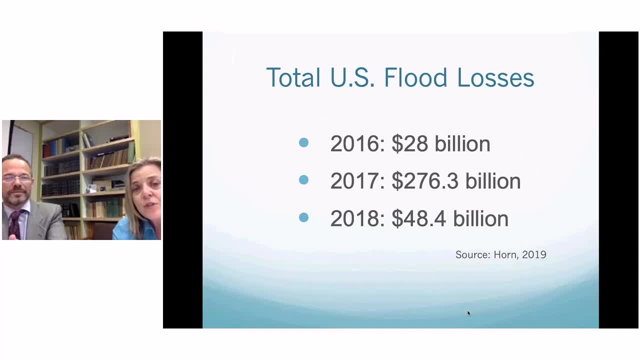 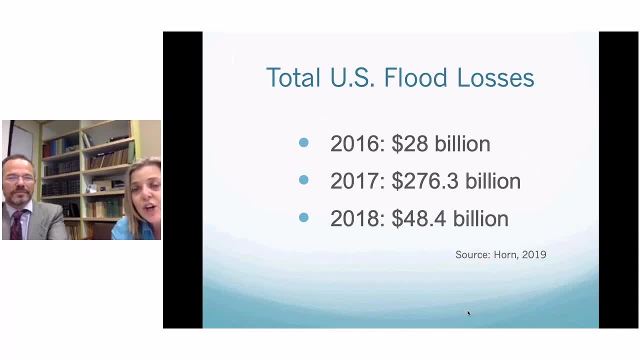 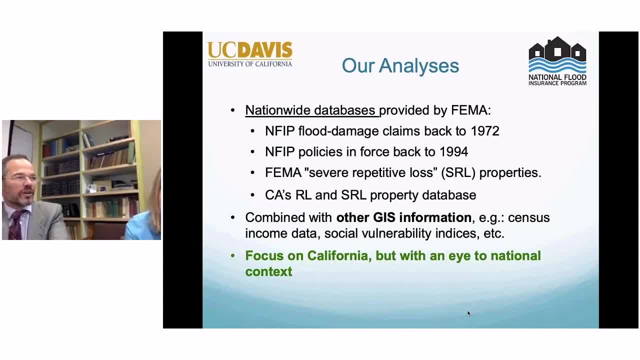 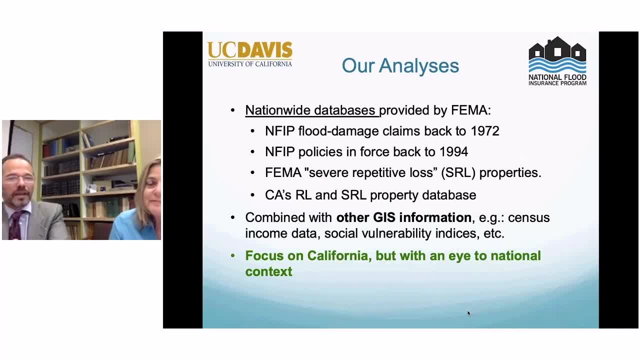 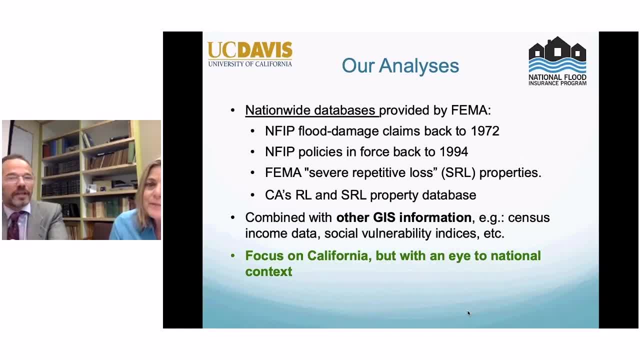 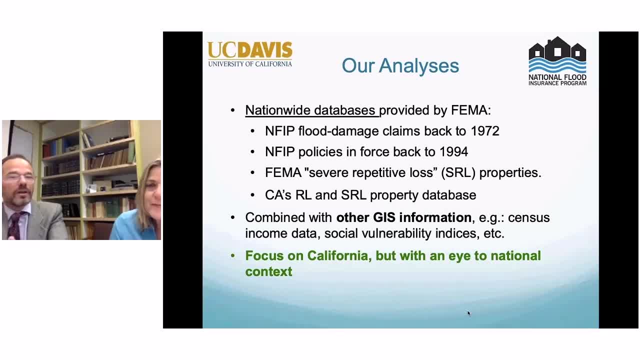 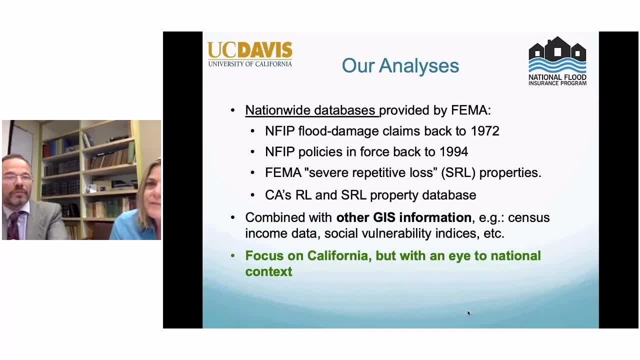 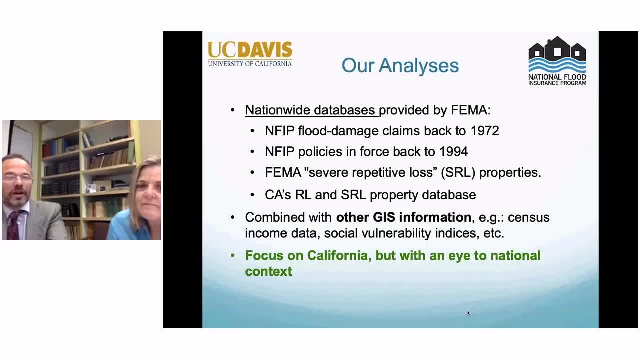 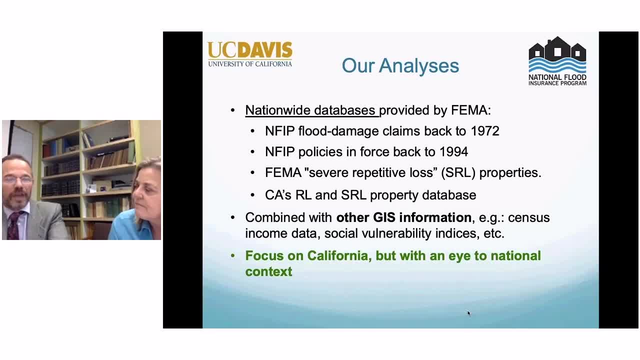 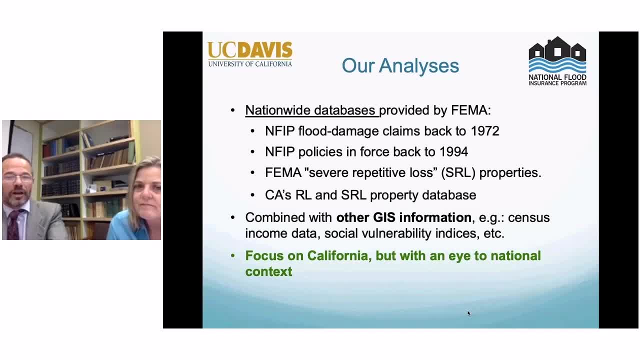 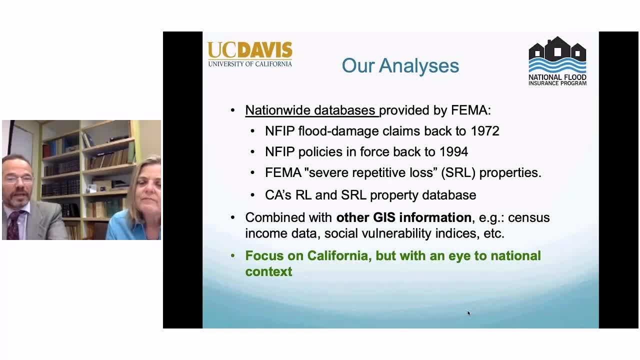 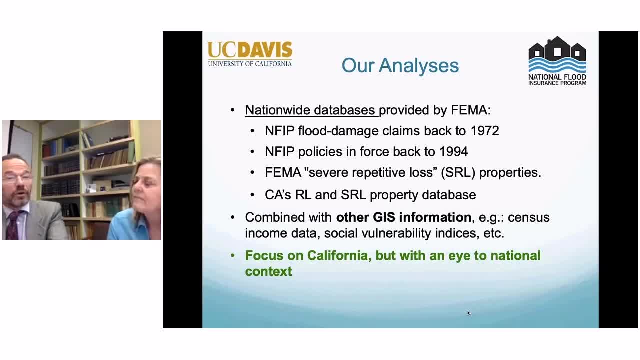 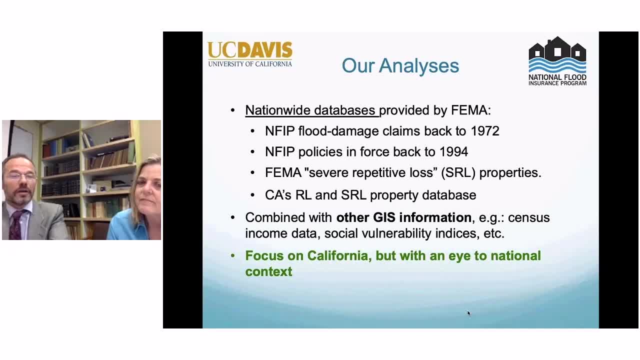 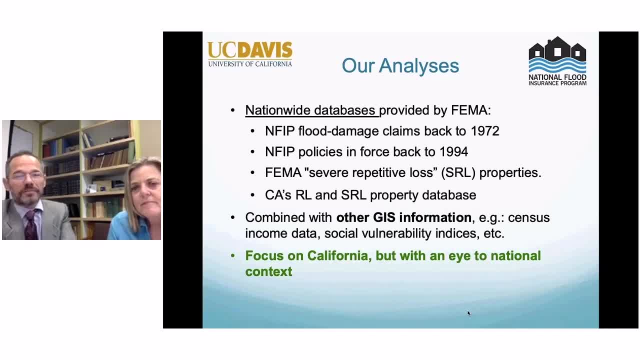 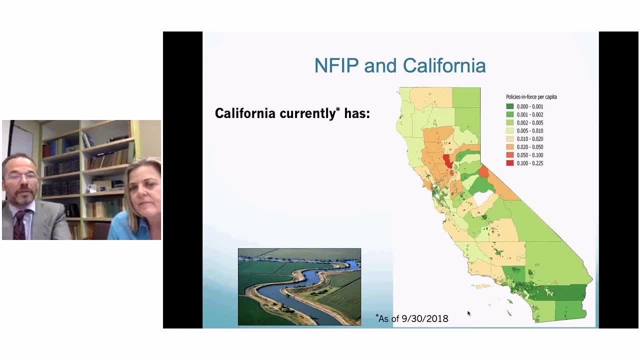 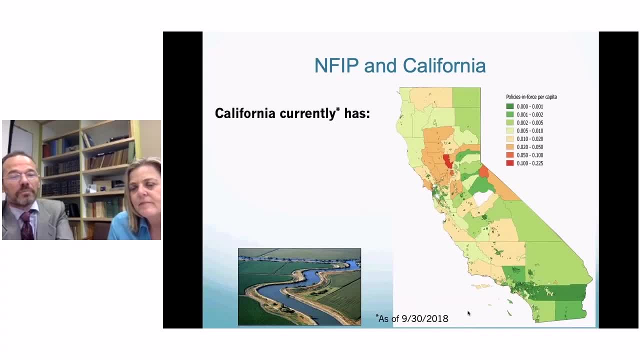 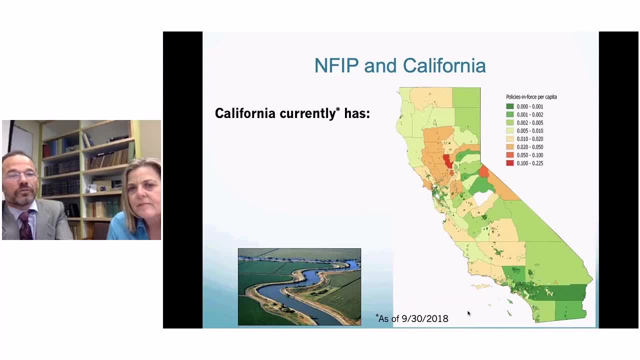 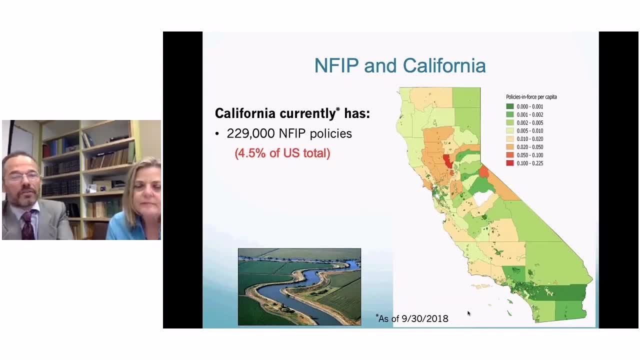 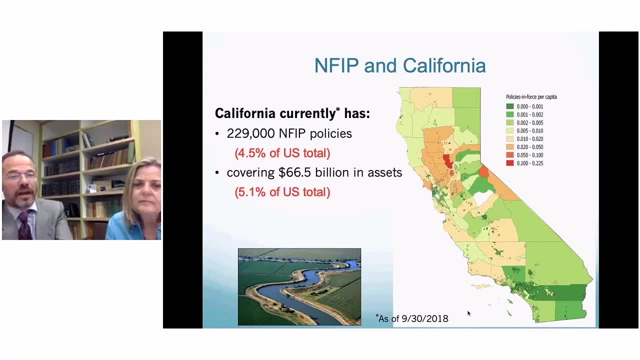 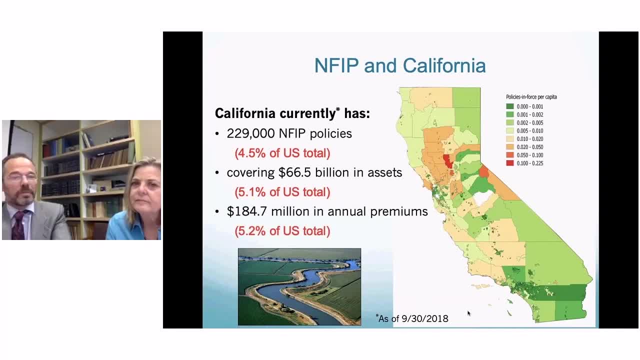 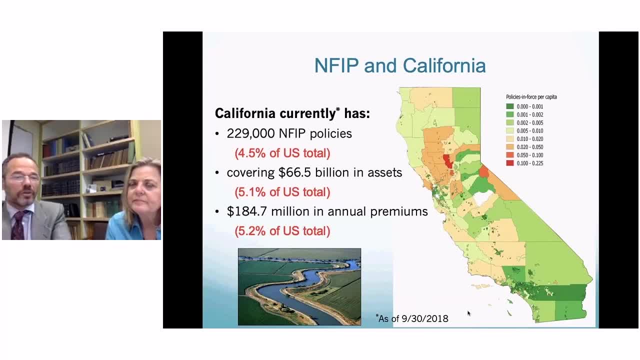 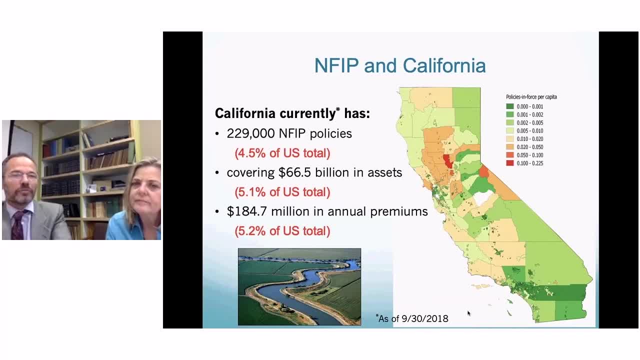 Diane also presented the current status of the flood losses, Clifford WuNowak. As a whole, California represents about five percent of the total insurance pool and expenditures —no, the total insurance pool, It's different. we'll talk about that- Five percent of the insurance pool for the nation. 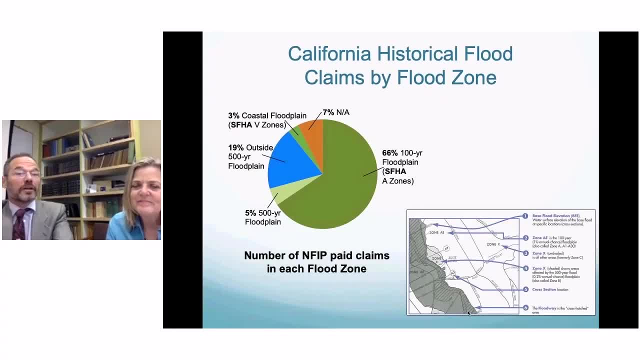 So, looking a little bit at the claims, the actual claims filed have been really interesting. This represents an empirical data set of actually where flood damages, flood insurance claims have occurred over a multidecade period And most but not all flood claims have occurred within the flood zone. 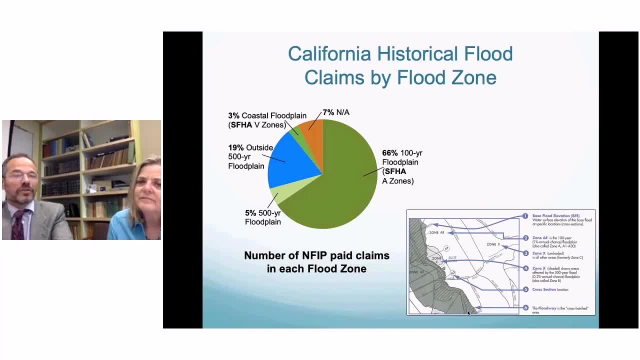 So others have commented on this. I'll call it. only about two-thirds of all flood claims occur within the mapped flood zone, That is, the 100-year or A-zone or equivalent flood zones. This is California data, right here. Some additional number- 20%- have occurred in what has been mapped as essentially the 500-year flood plain. 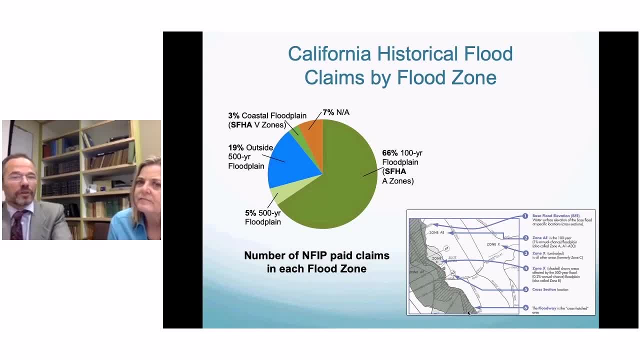 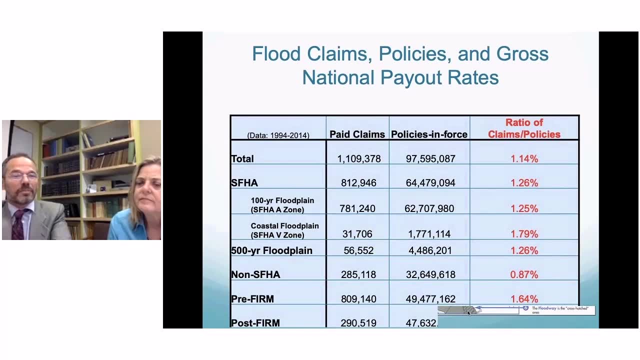 A relatively small slice of this pie, at least within California, has been within the mapped coastal, that is, the V-zone. Here are some of the numbers tabulating both claims and policies in force by different flood zones. There's lots of really interesting implications of some of these numbers. 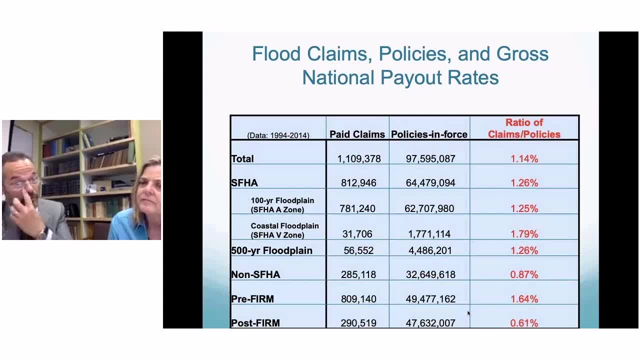 We don't have time to go into all of this, but I wanted to just highlight some of the sort of pressing issues we think for flood insurance, flood risk within the state. So one thing that jumps out of this particular tabulation is the relative balance between pre-firm 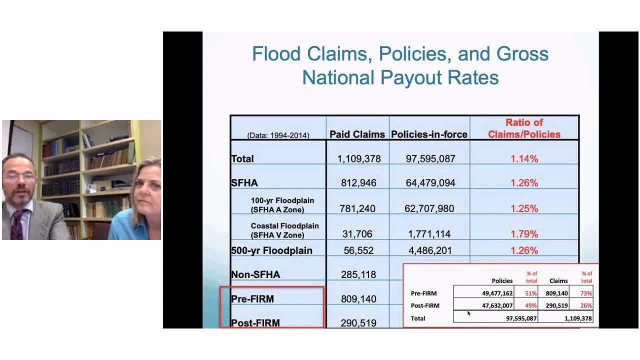 and post-firm policies and claims within the state of California. So pre-firm meaning most of you are aware of this- these are properties that existed before the first available effective map for any particular location. That's correct, Kathy, Yeah. 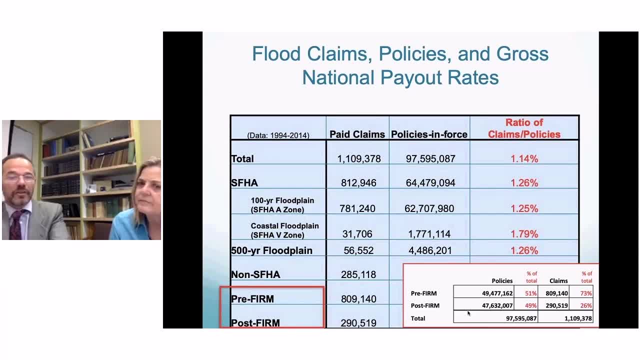 One of our initial hypotheses that I'll discuss later is that California maybe, was it was a newer state- had relatively little infrastructure that would be classified as pre-firm. that's mostly not the case. It's about 50, 50.. 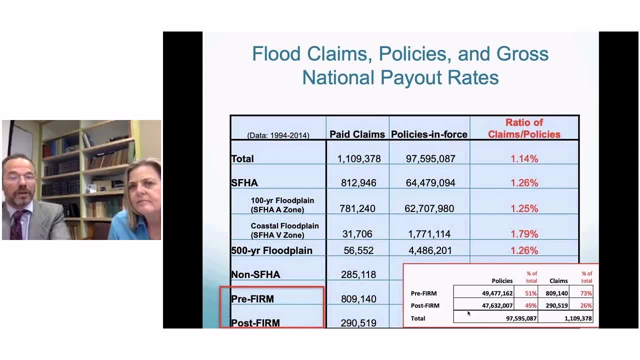 It's about 50% of California's NFIP policies- and this is over the history of the program- are on pre-firm structures And the other half- it's actually 49%- is on post-firm structures. Interestingly, and maybe not surprisingly, 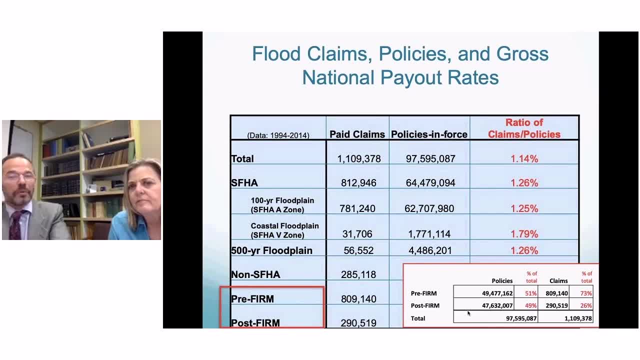 the pre-firm policies. the pre-firm policies of California are mostly based on pre-firm structures. Are those pre-firm structures have generated a disproportionate share of total claims. So, although they're about 50-50, 73% of all claims over the history of the program. 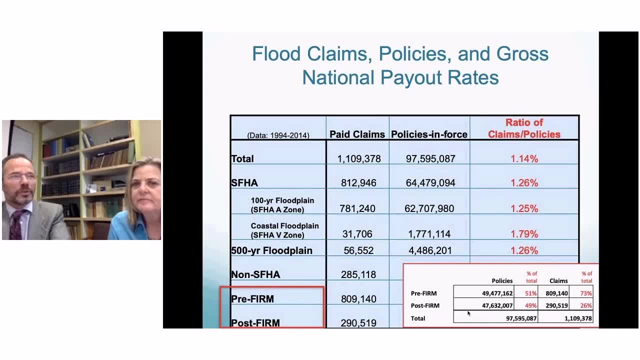 have been on the pre-firm structures. It's that disproportionate share that can be seen nationwide. Right now we're drilling into this a little bit further, looking at trends over time to see if maybe California is doing a better job or not. 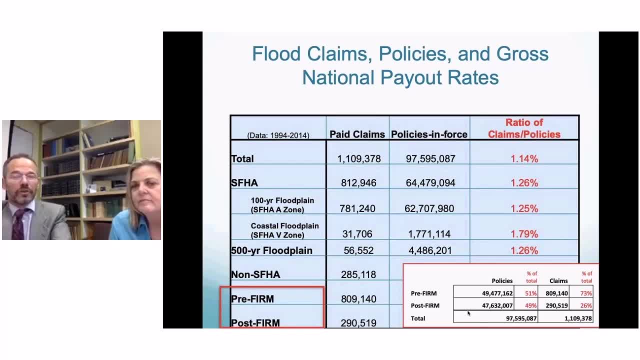 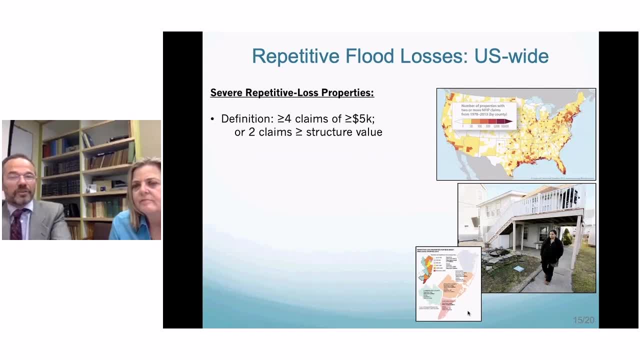 we'll see, of mitigating some of those early pre-firm structures. So something else that comes out of that is patterns in repetitive losses. So repetitive losses have been identified as a major challenge to National Flood Insurance Program and to really floodplain management in the US. 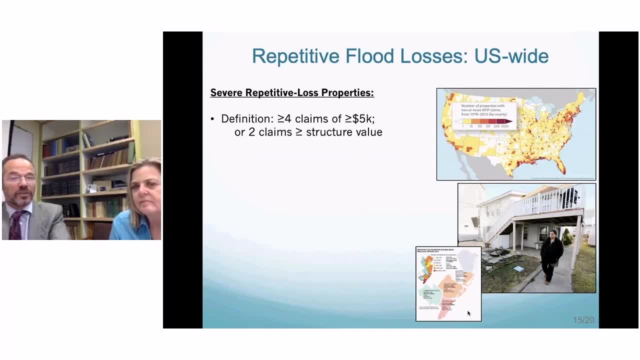 The initial idea of the program, as Kathy discussed in the 1960s, was to take on this risk but wind it down over time, reduce these roles of repetitive loss properties. There are again, as most of you know, repetitive loss properties. 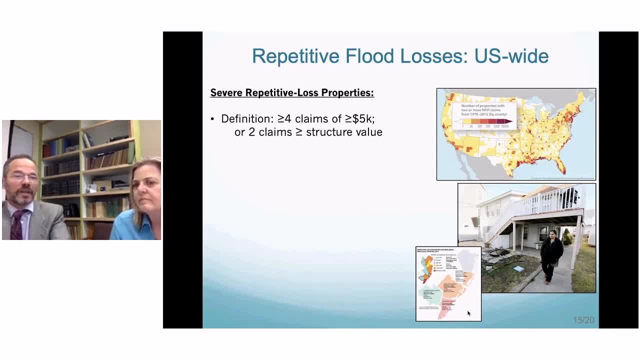 currently two formal classifications. The more extreme classification is severe repetitive loss properties defined as at least four, that is, four or more claims exceeding $5,000 in value, or two claims that total more than the structural value. And again, these are widespread across the country. 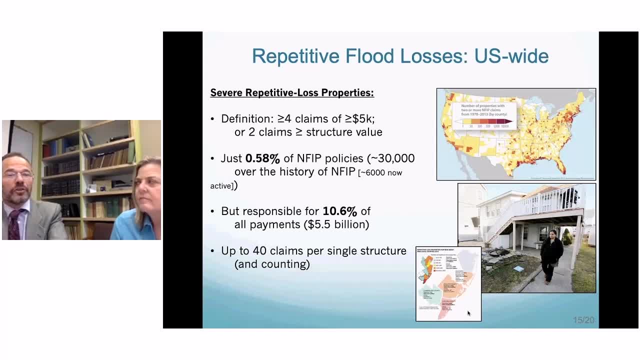 FEMA's total roster over the history of the program recognized 30,000 such properties. nationwide That represents 0.58, so a little bit over half of 1% of total NFIP policies over the history of the program. But that half of 1% of policies has been historically responsible. 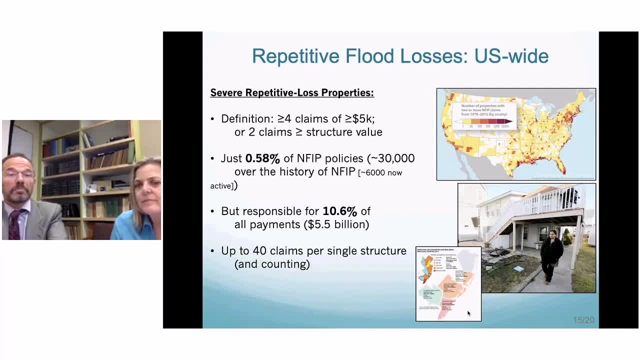 for well over 10% of all NFIP payouts, So something like a 15% to 20% disproportionate load on the program in terms of dollars expended. That list of severe repetitive loss properties is a rogues gallery in any floodplain manager's book. 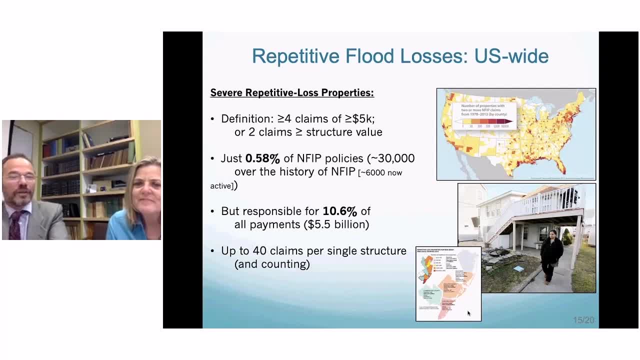 In that roster the worst single structure had received 40 different payouts on the same structure, rebuilding each time just under, apparently, the recent 50% threshold by which that owner would have to mitigate Another structure, and we've mentioned this to a number of different people. 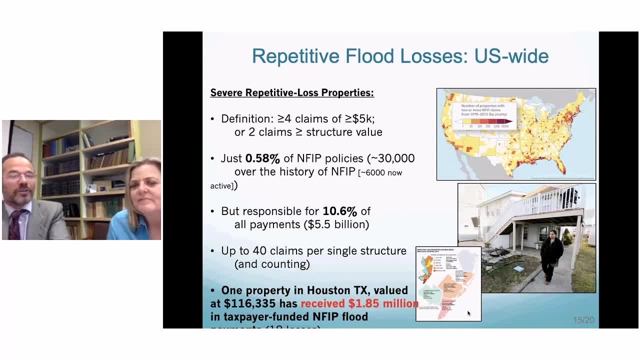 in Houston, Texas, was valued at $116,000, but has received a total of $1.85 million in taxpayer payments to rebuild in the same spot, And that's 18 separate losses. So this is any insurance agent's nightmare scenario. 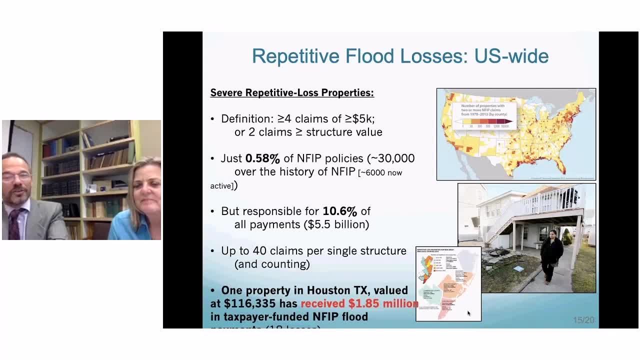 And probably no private insurer would take on this policy. That's the nature of NFIP, the insurer of last resort. So just to focus that on California a little bit, California's roster includes- and this is over the history of the program. 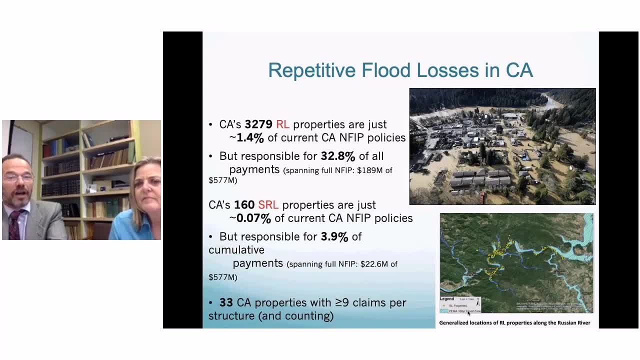 3,279 repetitive loss properties, some of which have now been mitigated. But over the history of the program, that 1.4% of all policies has been responsible for a striking 32.8% of all payments. really a very striking, disproportionate share. 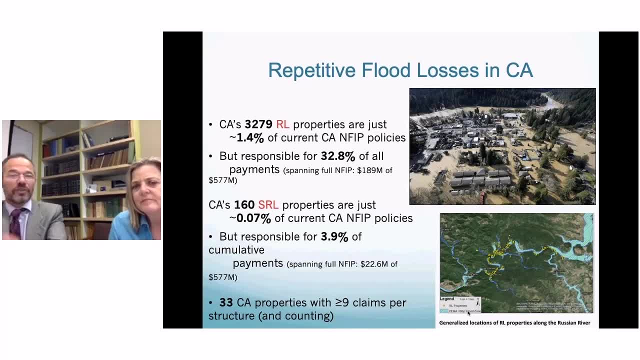 of all NFIP payments in the state of California. So again, we're looking at right now. looking at right now some of the trends, whether this has gotten better or not. California has a relatively small share: just 160 severe repetitive loss properties according to the data we analyze. 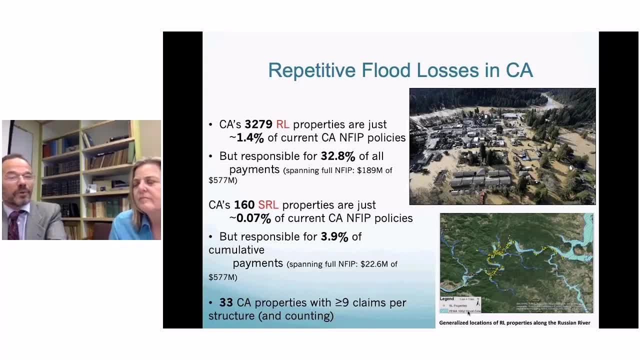 but again this represents something like 0.07 percent as a proportion of current NFIP policies within the state. but over the history of the program that 0.07 percent severe repetitive loss properties within the state has generated a wildly disproportionate- roughly four percent of cumulative payments over the history of 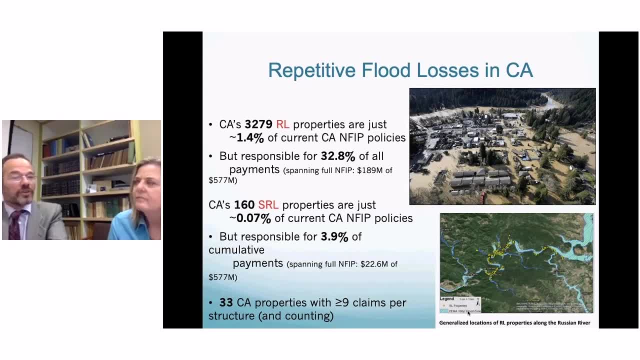 the program Based on the roster, we see 33 California properties with at least nine repetitive losses, and that counts as severe repetitive losses in most cases on those properties. and this doesn't count February's flooding on the Russian river. so we suspect many of these properties have added one more to 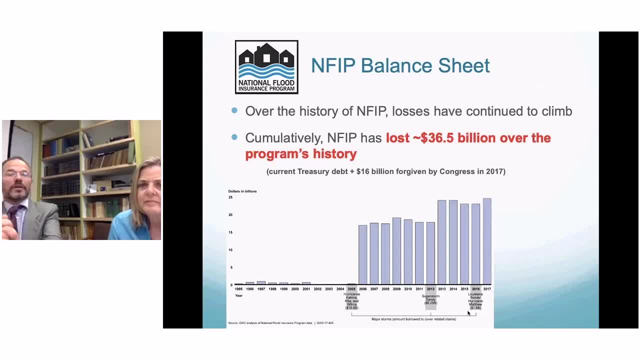 that count. So again, bouncing back to the nationwide picture just for a moment. over the history of the program, losses payouts have generally exceeded the total cost of the program, have exceeded the premiums collected the the income to the program. This has occurred mostly in in a couple of major jumps, most most pronounced, 2005, which was hurricane Katrina and other events concentrated on the Gulf of Mexico coast. If you add up the total imbalance, the insurance on that debt which continues to accrue, and add in 16 billion dollars forgiven by congress in 2017, by that count we tabulate that NFIP. 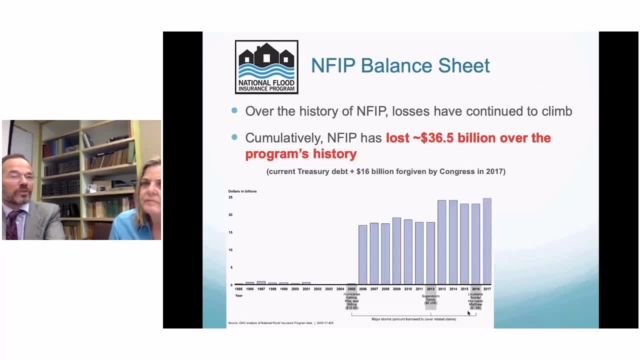 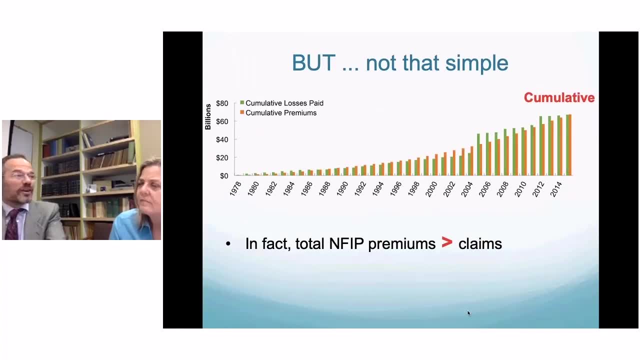 has been a 36 and a half billion dollar money loser to the federal government, to the federal taxpayer, over the history of the program. The picture is not entirely that simple, though, that if you simply look at the dollars paid out in losses to policyholders compared with the premiums paid in by 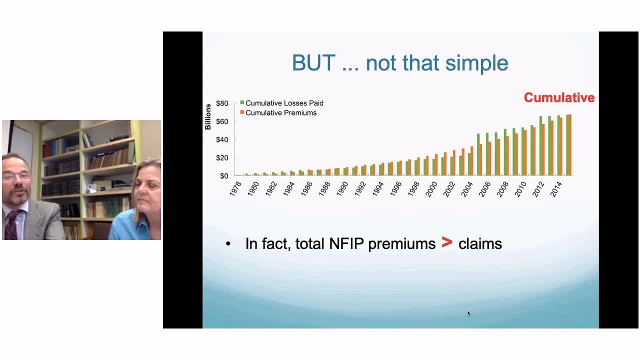 those same policyholders. by time as of 2015, at least, the premiums exceeded the claims. I think that has tipped slightly in the opposite direction in 2017, with a couple of big payouts. But the issue is not just the imbalance between incoming premiums and outgoing payments. The issue- and this has been identified by a number of government agencies- is the additional fees, in particular 34 percent of fees taken out of premiums for the private insurers under the write your own- write your own policy program. So this has been identified as a significant drain on NFIP's resources and in recent 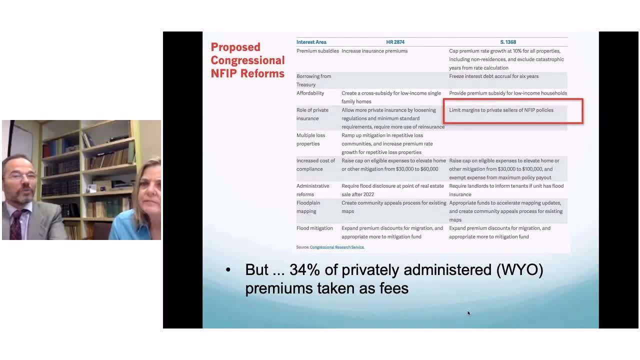 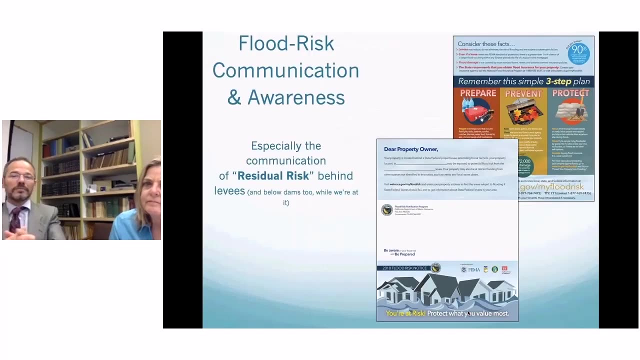 discussions, which maybe we'll have time to talk about, recent attempts to reform and reauthorize and extend the NFIP. this issue has been highlighted, at least within the senate version of the reauthorization and reform bill, as something that needs to be addressed. One other issue that our group would like to highlight: 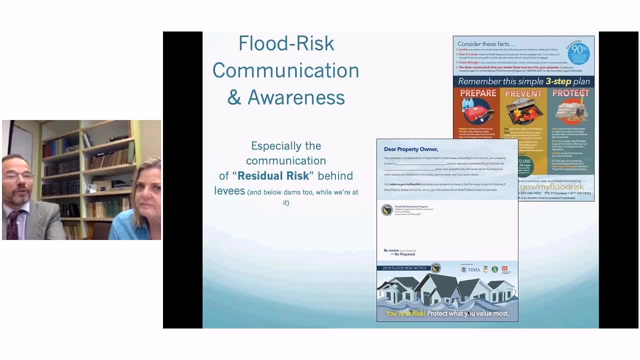 is the continued challenge of flood risk awareness, or usually the challenges lack thereof, and this is in california and nationwide. we could talk about this. I would suggest we would suggest that california actually does a pretty good job of getting the word out, or doing its best to try to make its 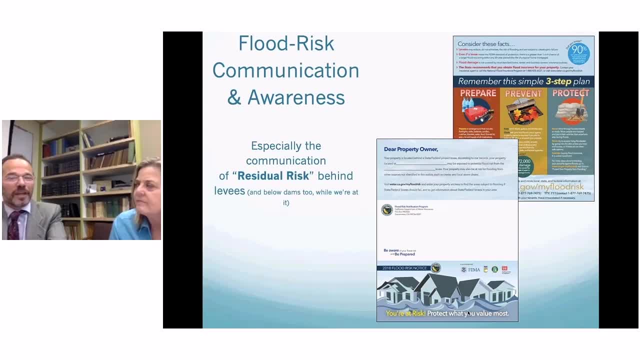 its residents aware of flood risk they they may be facing. So this is what we believe to be the most the most recent flood risk notice distributed- Our understanding is this is to residents covered by the central valley, by the central valley flood protection system. Sorry, we're mangling the exact terminology here. 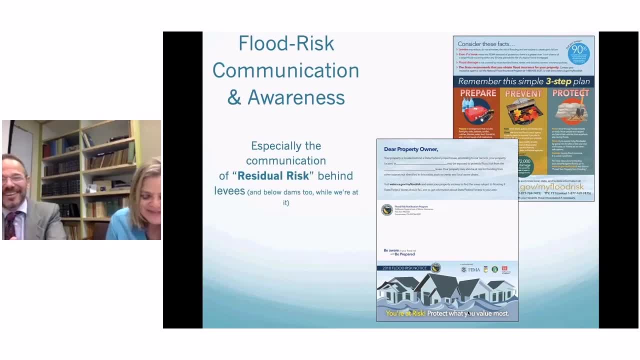 The state plan of flood control. There you go, There you go, Thank you. So this is this is a a good step in the right direction, but I think most people would agree, not the only step that needs to be taken. There are continued challenges. for example, we would highlight the continued challenge. 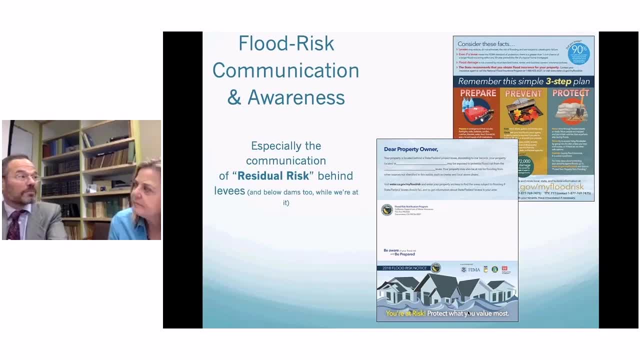 of residual risk behind levees and behind dams as well. In addition, we would point to the possibility of using catastrophic risk models for flood awareness, as well as as well as other applications. So some of you may have seen the excellent tool. This is temblornet that currently provides individual 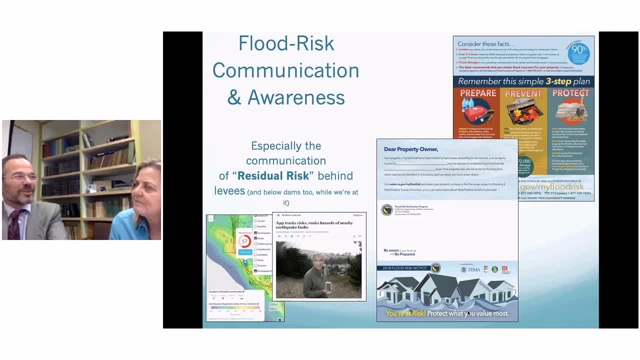 flood assessments- Sorry, not flood assessments. This is seismic earthquake hazard assessments, individual properties. you can plug in your own home address into this and it'll tell you what your risk is and annualized over 30-year mortgage and the effectiveness of different mitigation tools. 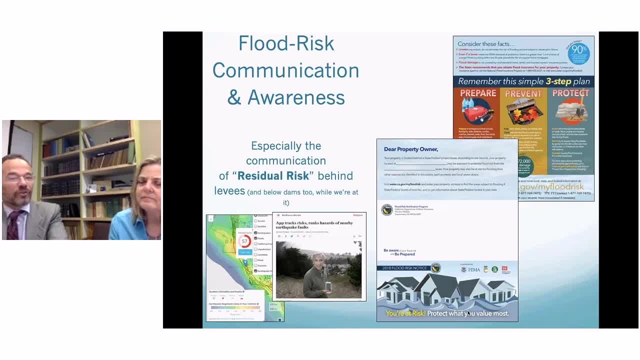 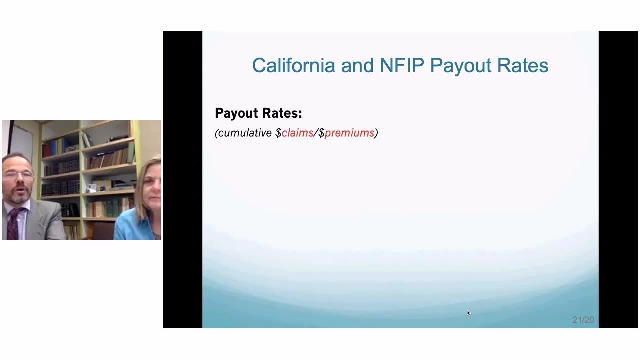 So some of you are aware that we at UC Davis are trying right now- we have a proposal pending- to partner with temblor and to do for flood risk, and actually for wildfire risk, what temblor currently does for seismic risk. What we'd like to highlight quickly now is some of our analyses focusing 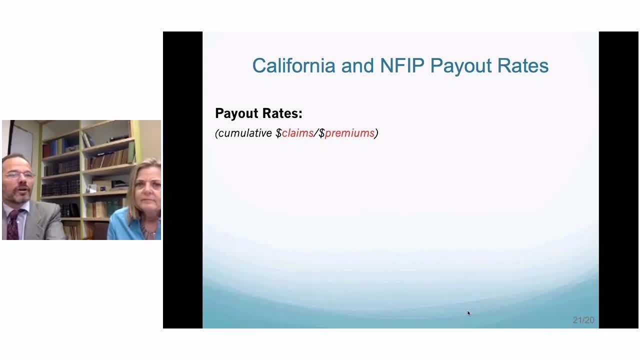 on this number, what we call payout ratio or payout rates here, and this is a ratio for different jurisdictions, different intervals of time of NFIP claims or payouts versus NFIP premiums, which is the income to the program, again for any given jurisdiction or unit of time. 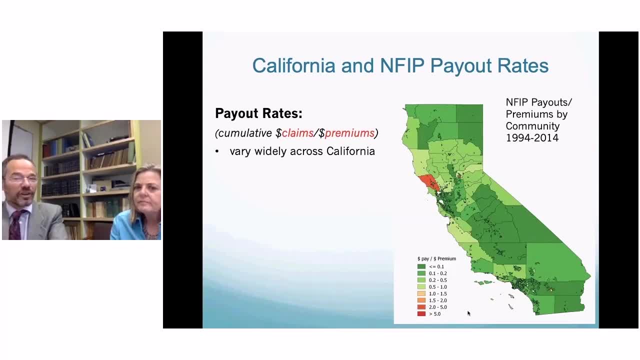 Looking at California, what you can see is that this ratio varies widely and wildly. So that is the number of years that we are talking about in this slide from less than 10%. in fact, a lot of California is zero on the scale over the. 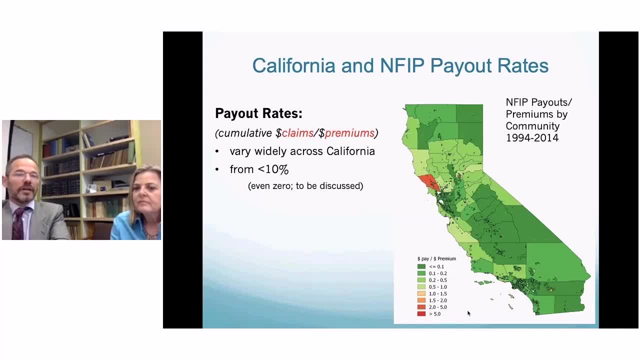 period of time that we analyzed. so less than 10% means less than a dime of pay outs for all the insured properties within that jurisdiction over the history of the program. for each dollar that that jurisdiction is paid in in premiums, that goes to over 500% for California, and so what you can see are: 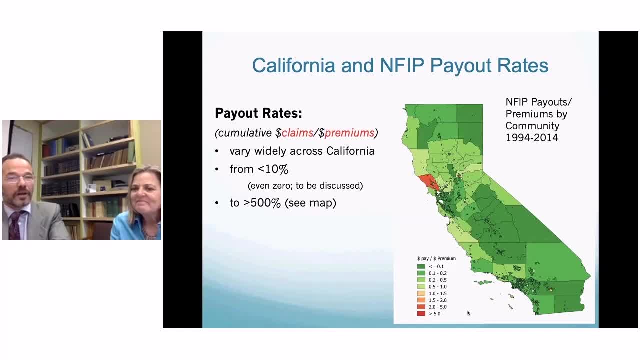 small but distinct areas with claims that have significantly exceeded premiums over the 21 year period of time that we that we studied. however, the overall picture is that the majority of California is is green. in fact, the the big takeaway of this analysis, which was I opening to us at the time, is that, since 1994, NFIP damage payouts within the 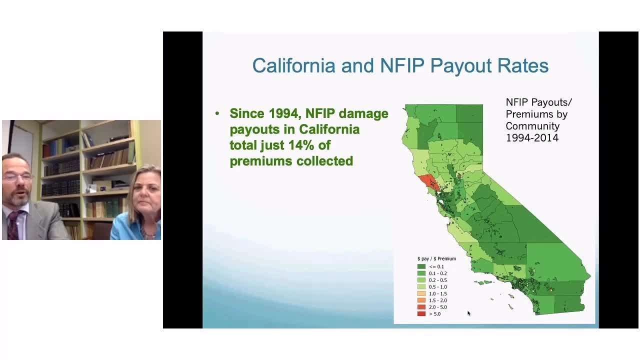 state of California have totaled just 14 cents per dollar premiums collected statewide, although again that that varies a little bit by region. so if you tabulate, accumulate that, that imbalance over that 21 year period and just for inflation it totals over three billion dollars of net outflow. 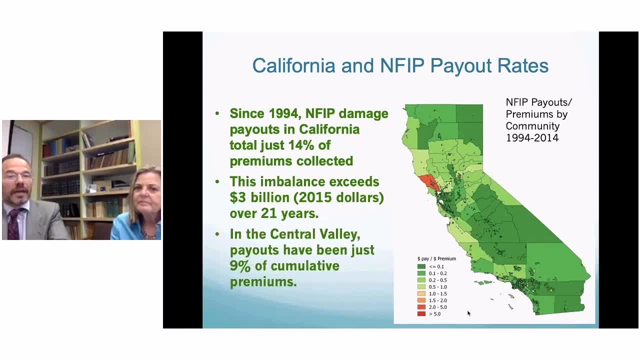 from the state of California and in localized areas, for example the Central Valley. many policy holders are aware of this imbalance and have complained about it and brought attention, for example GAO study, to this issue. the ratio is even worse for the Central Valley, and that's not even separating out AG policies from residential policies, the, the. the total is just nine cents of payout per dollar premium going into NFIP. so, looking by count of jurisdiction, statewide, ninety-seven percent of California jurisdictions have paid more, most cases substantially more- in premiums than they've received in payouts, and in fact twenty-two percent. 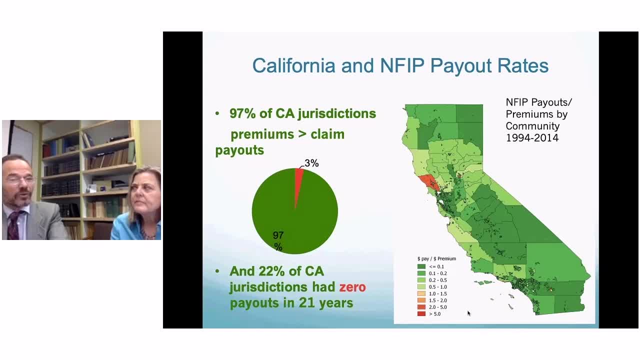 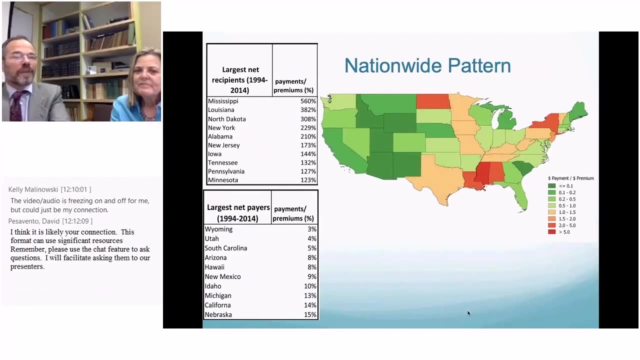 of California jurisdictions have had zero payouts in the 21 year period that we studied. we would love to update this database if any partner would like to help us get the updated date data from FEMA. data from a qualified fiscal officer that will be showing, but no additional. 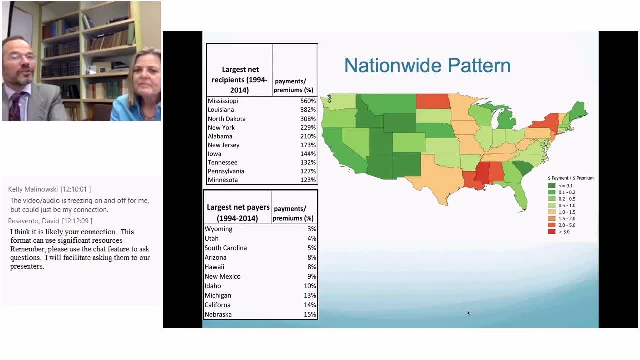 information. Thank you. For example, in the case of Michela, California is the only state in green in state of California. California is the only state in green in its own state. so California is not the only state in green in its own state. So just to put that pattern into a national perspective, California is not. the only state in green. Nor are we the most extreme example. again, California, having received fourteen cents on the dollar Back in terms of at least a disaster payouts, has received $5.60 in disaster payouts alone for dollar premiums they've paid into the program. 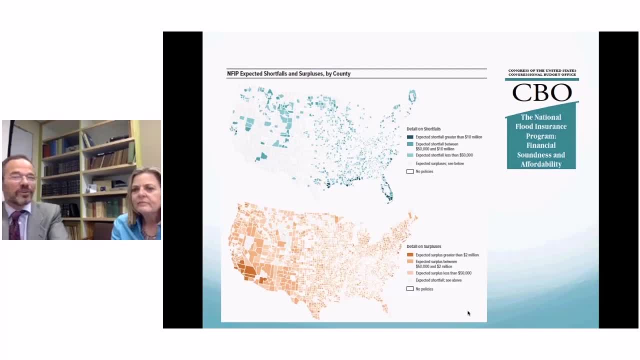 So we began making noises about this. This is already back in December of 2016.. I suspect as a result- direct result of the noise coming out of California- this has been brought to the national attention. Congressional Budget Office has looked at this and echoed that finding. 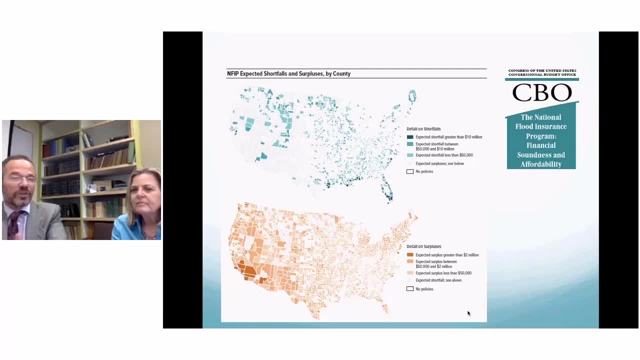 in a report that we're happy to share with anyone who's interested. They've mapped out both the net shortfall- what we would call the net recipients- and the net surpluses- the net donor jurisdictions- on a nationwide basis, And this is an interesting couple of maps. 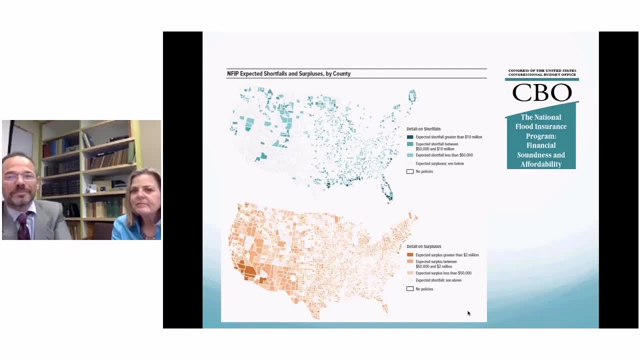 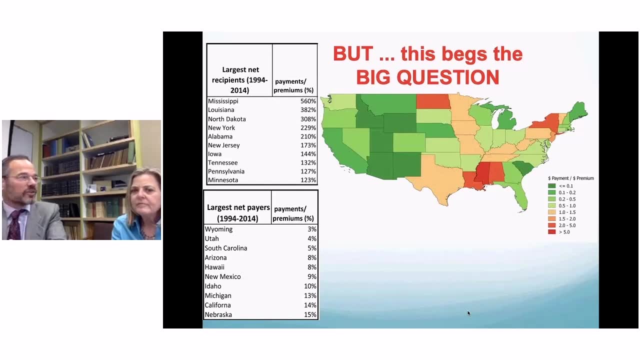 Happy to talk about this more if time permits. But looking at what this implies for California, what we here at UC Davis suggest is there is one first and last And the most important question that needs to be addressed, And that is over the last 20 to 30 years. 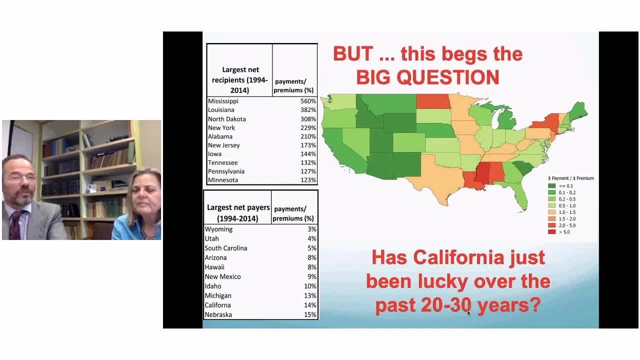 of available record, that is most of the history of NFIP. has California really just dodged a bunch of bullets that other states have not? So at least on the other extreme, some states are on that rogues gallery, that worst case list, because of a single event. So, believe it or not, Louisiana. 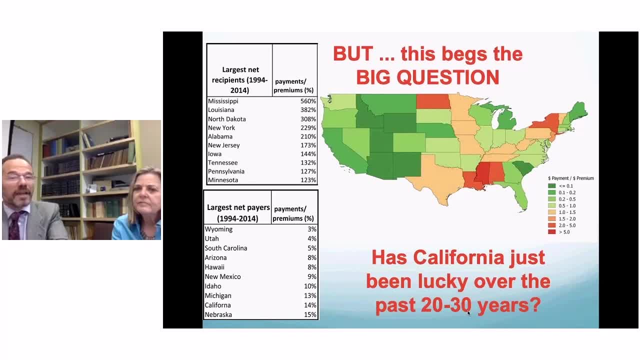 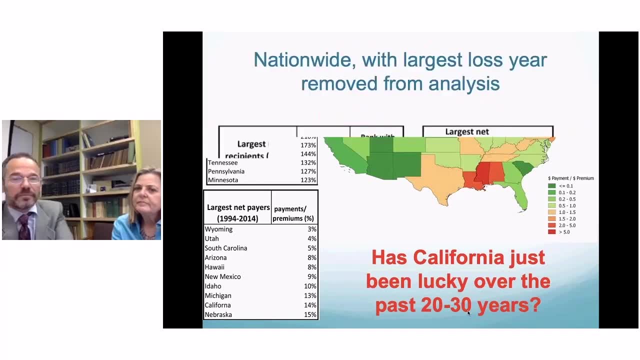 was a net payer into NFIP And that's a very important question. And that's a very important question because we've been looking at this data since 2005, until Katrina hit And that tipped the balance of that one single event. So we've attempted to analyze that one-off situation using the available 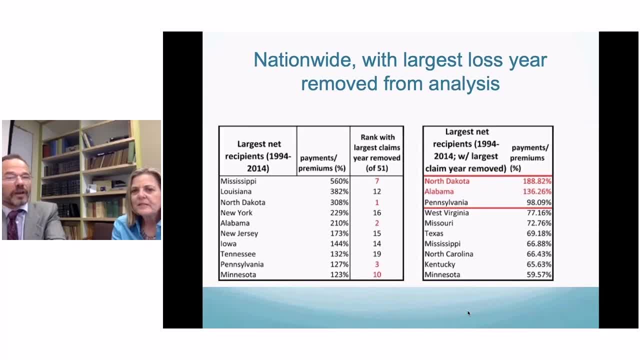 data by taking the single worst loss year out of every single state's record and just seeing how that changes things. And so, for example, Louisiana, which was number two on the list of net recipient states, dropped significantly down to number 12 on the list. 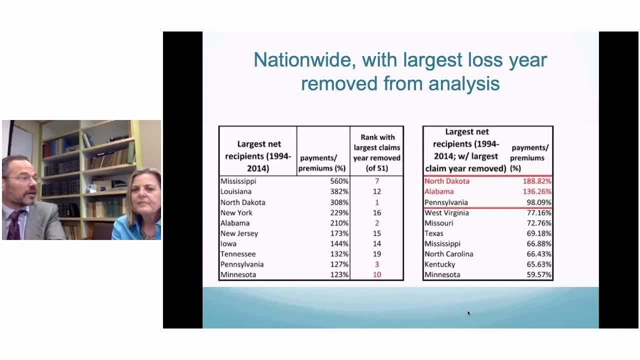 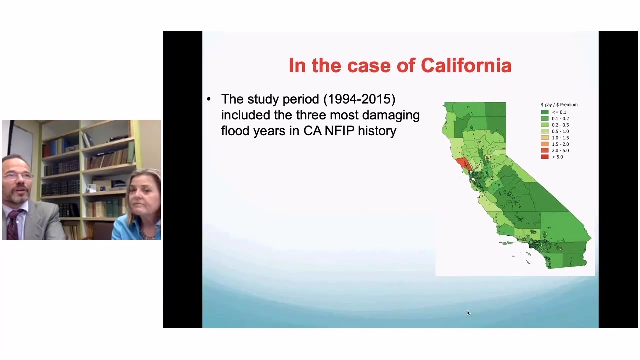 New York and New Jersey are the same thing because of Hurricane Sandy. Other states as illustrated on the right there. even when you take out the worst single year, they still remain pretty significant net recipients of NFIP funding. So that remains, I would suggest. I think Kathy would agree- an open question. But we here in California would suggest you look at at least a couple other considerations. looking at the state's track record, That study period- 1994 to 2015,- included the three most damaging flood years in California NFIP history In only one of those years only, in 1995,. 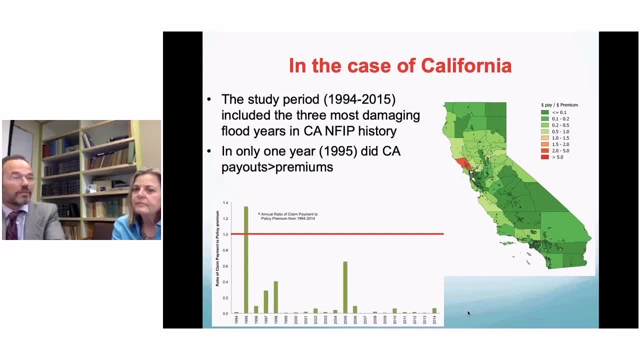 did California's payouts ever exceed the premiums? And even so, just slightly. So even in that worst single year of recent history, it was something like $1.30 of payouts for the dollar paid in, And every single other year California paid in more in premiums than 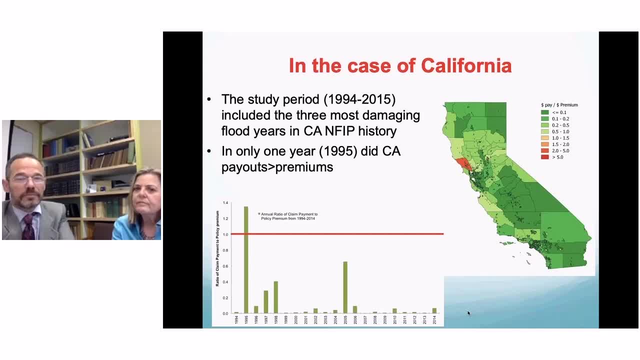 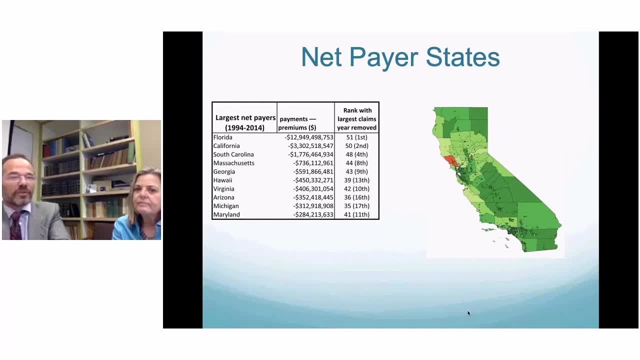 it got out, at least in terms of disaster payouts from NFIP. So again, as already mentioned, sort of the big takeout from this is that when you add that up, and that's just over those 21 years, the total adjusted for inflation is: 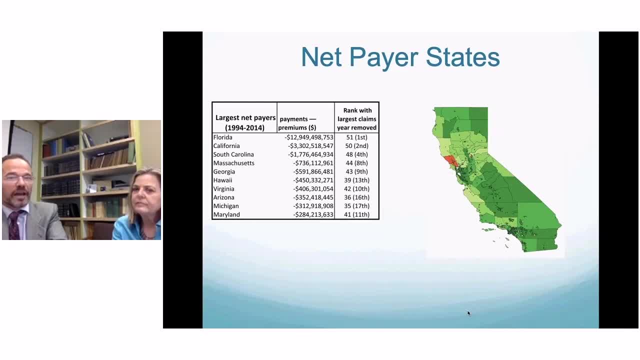 $3.3, actually $3.3 billion of net outflow, California essentially subsidizing over that period of time the net recipients on a nationwide basis. We're not the only ones. The number from Florida is even larger and, I would say, very interesting on its own. another worthy discussion. 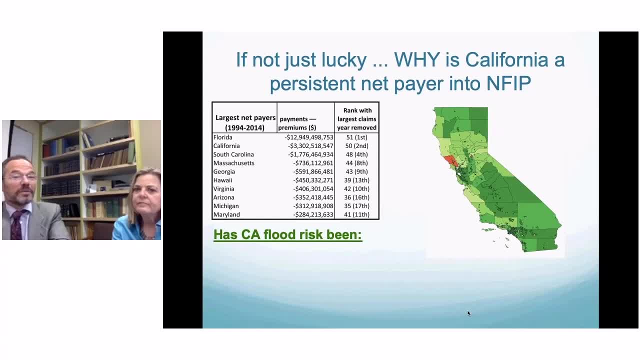 But this opens up some other questions that need to be asked. So if California, if hypothetically California has not just been lucky, what other potential facts, factors could be making California and some of its other states net payers into the program? So again we ask these questions: Has California flood risk perhaps been? 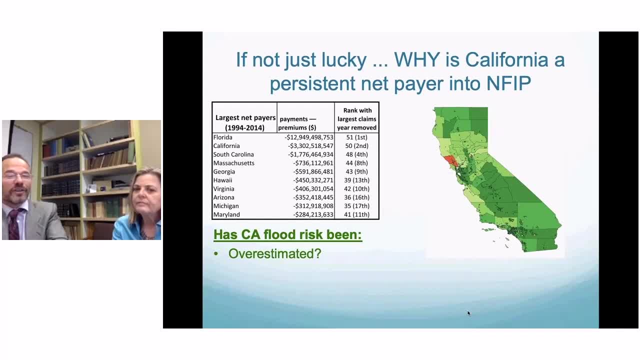 overestimated. So Kathy is going to talk in just a minute about the nature of flood mapping, FEMA maps in the state of California, Some other things we've looked at again. one of our initial hypotheses was the nature of pre-firm versus post-firm building stock. 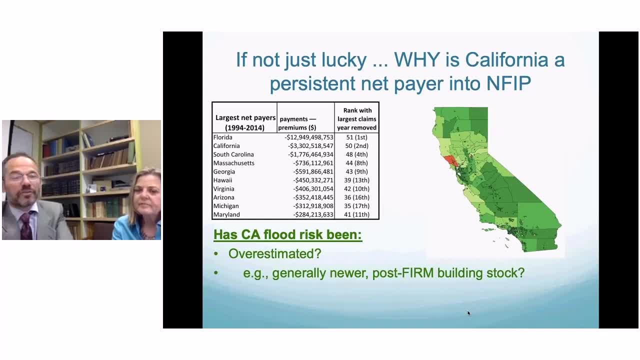 Within the state of California compared to other parts of the country. One thing that we're very interested in- and having some trouble getting good data on- but we're doing our best- is: has California managed and perhaps mitigated some of its flood exposure more successfully than other areas of the country? 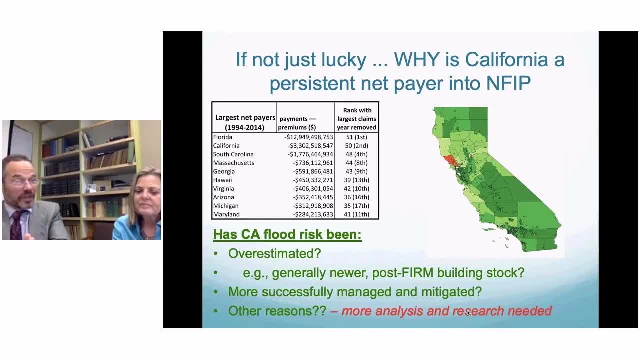 Or a wide range of other potential reasons, mechanisms, for sure, more analysis and research needs to be done. Sorry, that's always a conclusion a researcher makes, but I think it's absolutely true in this case. So, again, one thing that we are increasingly focusing. 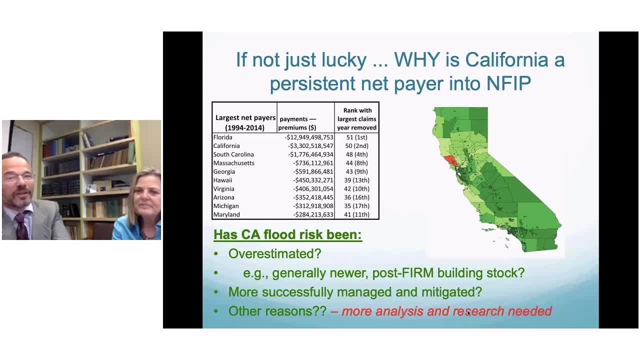 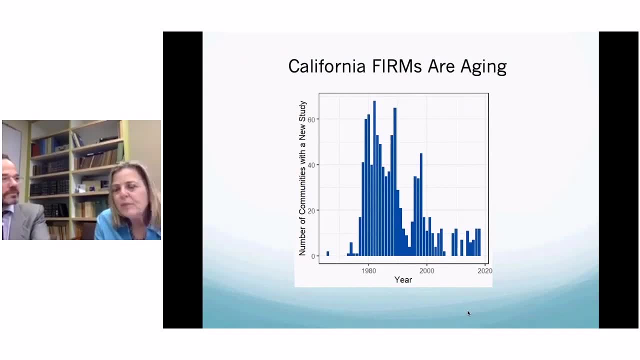 on, in particular because of some analyses Kathy has been doing, is on the nature of flood maps within California. So one of the things we find is that many people don't realize how old many of the studies within FEMA that make up the FEMA maps, how old they are. 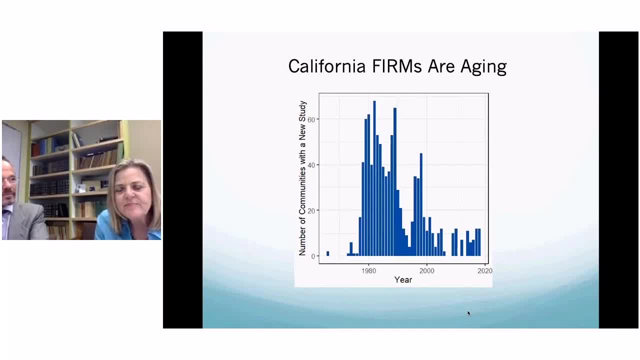 California's flood insurance rate maps are aging. I recently completed a study where I looked at the age of all of the maps, all of the FEMA initiated studies and you can see from this chart that in the late 18 and 1980s and early 1990s. 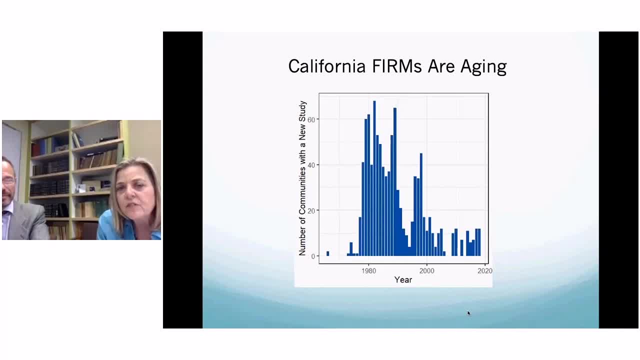 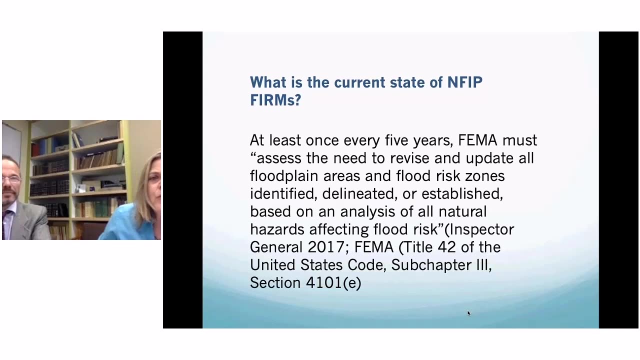 there was an influx of California studies, of effort to get the map program up and running, and then, with time, the number of new FEMA initiated studies has declined, and so, as we see, our maps are aging, and so the question becomes: what is the current status of the NFIP flood insurance rate maps? 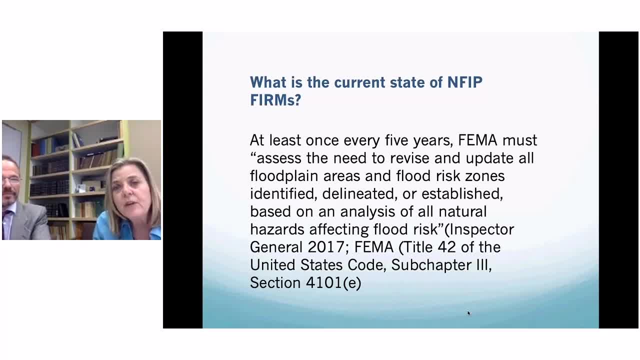 Well, by law, Congress has mandated that FEMA must assess the need to revise and update their maps, and the process that FEMA uses in the term is to provide a map of the flood insurance rate maps and then to provide a map of the flood insurance rate maps. 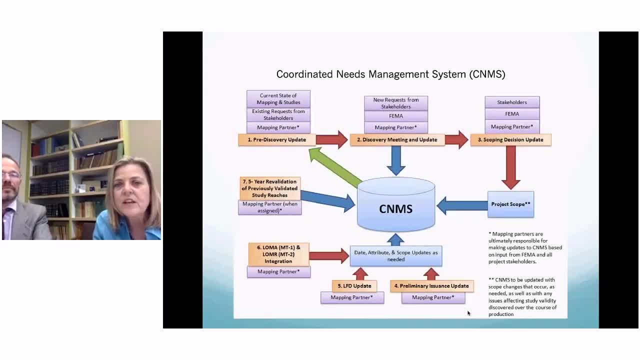 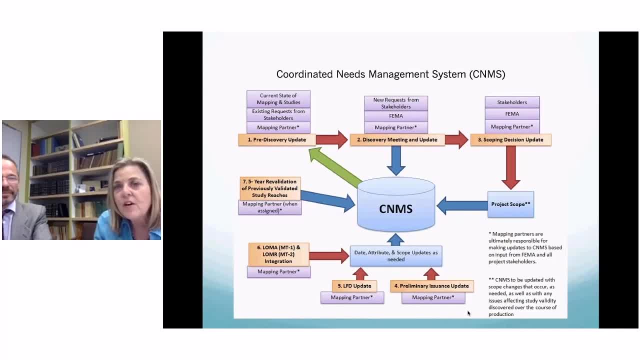 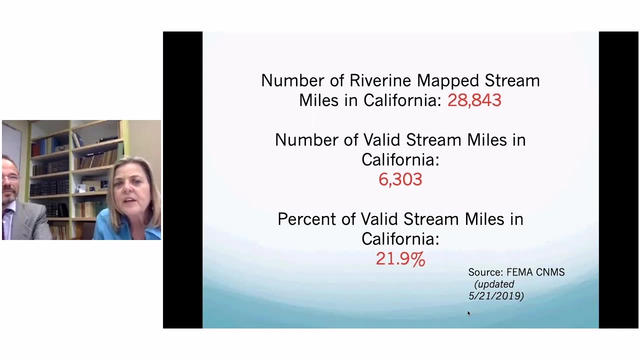 The CNMS. through the CNMS system, the stream miles are evaluated against a set criteria that's spelled out in detail at in the CNMS technical reference guide. The CNMS system has shown that the number of map stream miles in California totaled slightly less than 29,000. 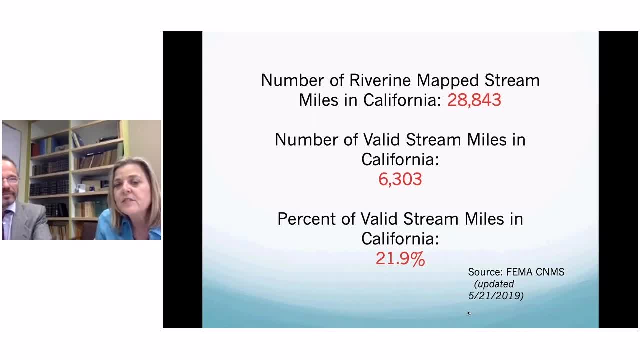 But of those 29,000 map stream miles in California, FEMA, through the CNMS system, rates only slightly more than 6,000 of them as valid. In other words, only 6,000 of the 28,000 meet all of the criteria that FEMA has identified for a stream mile to be identified as valid. 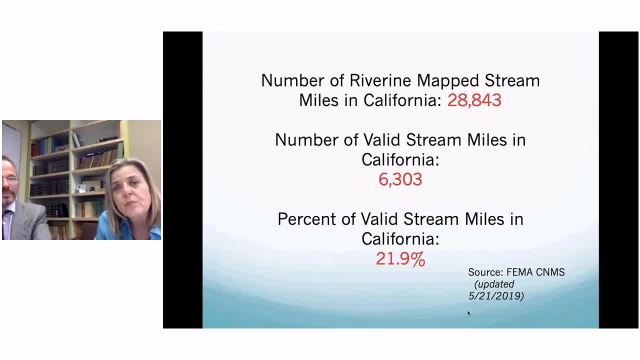 In other words, only 6,000 of the 28,000 meet all of the criteria that FEMA has identified for a stream mile to be identified as valid. So as a result, we have 22% of the stream miles in California by FEMA standards. 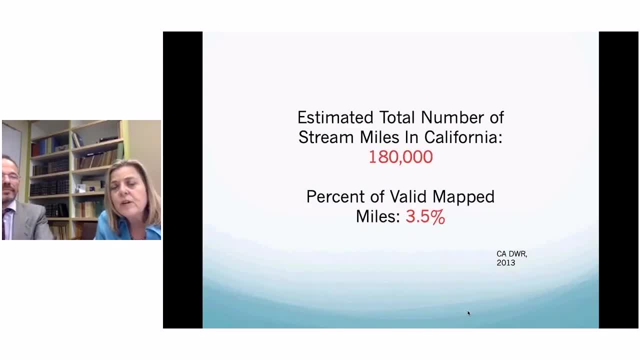 are considered valid. In 2013,, the Department of Water Resources conducted a study for FEMA and in their study they estimate that california has 180,000 stream miles. So if you do the math, comes out to say that only 3.5. 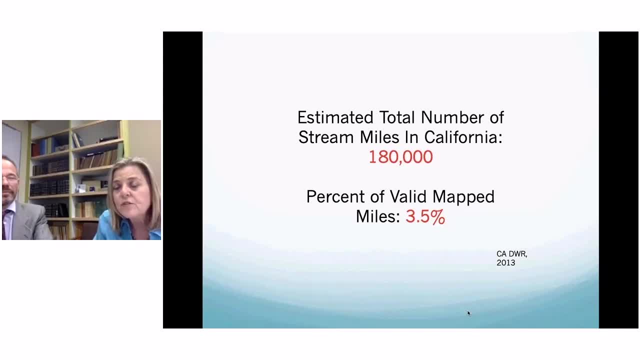 miles of the total California stream miles- 3.5%, thank you, 3.5% of the total stream miles in California have a valid FEMA map. So the next question then comes is: what will it cost to update the FEMA maps using the current risk map process? 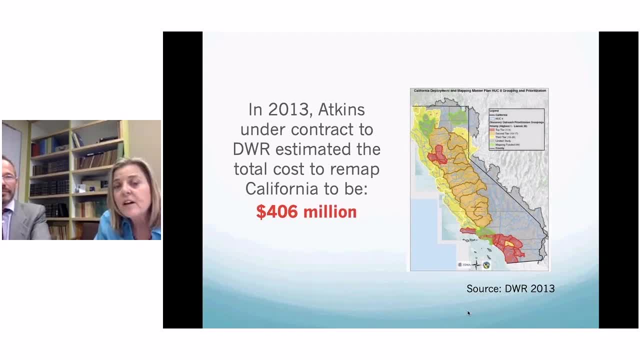 Again in 2013,, FEMA contracted with the Department of Water Resources through a cooperating technical partner grant to assess the state of the FEMA maps and to assess what would it take to map all of the state of California using the FEMA risk map process. 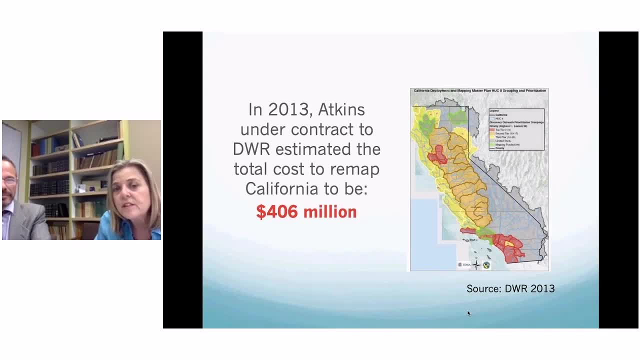 Atkins, under contract with DWR, conducted a very detailed study and found that the total cost to remap California at the time using the FEMA risk map process outlined at the time in 2013, was going to cost $406 million to remap California. 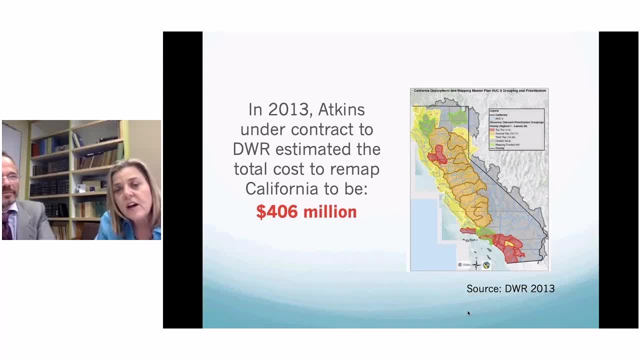 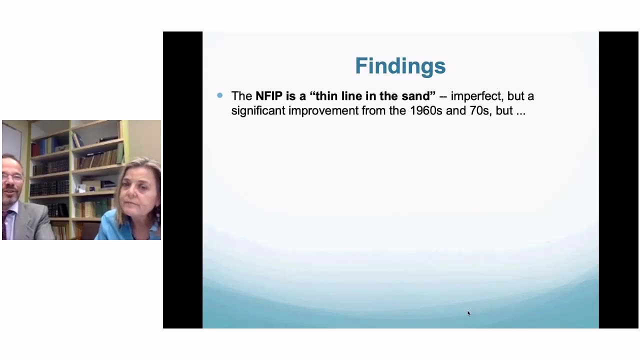 So the takeaway from that is that unless budgets change or the process changes, there may be many communities that will never again see a FEMA map. So just to move our way, So just to move our way towards conclusions here, we'd like to tip our hats to National Flood Insurance Program. That NFIP was an enormous improvement upon the situation that preceded it through the 50s, 60s and into the early years of the program- the early 70s- spiraling losses and unfettered floodplain development were the law of the land. 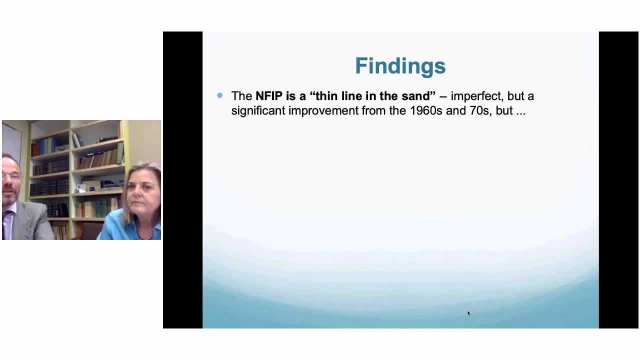 FEMA was a distinct improvement upon that, but it remains a thin line in the sand, imperfect, It's a perfect solution and we struggle with its imperfections today. Among those challenges, FEMA maps in California, and I think this is a pattern nationwide. 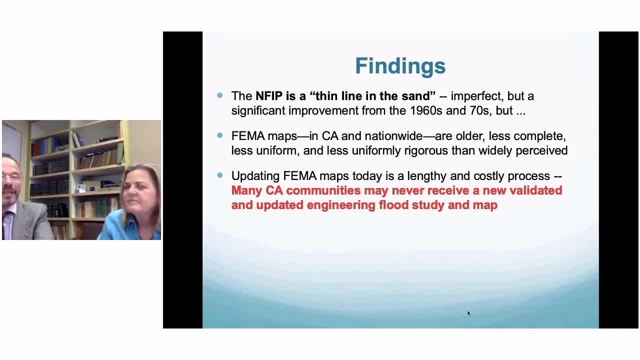 these maps are older, they are less complete, less uniform and less uniformly rigorous than widely perceived. So the last minute preparing this PowerPoint, we were pulling up pictures of computers as they were being used And we found that they existed during those early studies and, if anyone remembers, 5, 1⁄2 or 8-inch floppy drives. 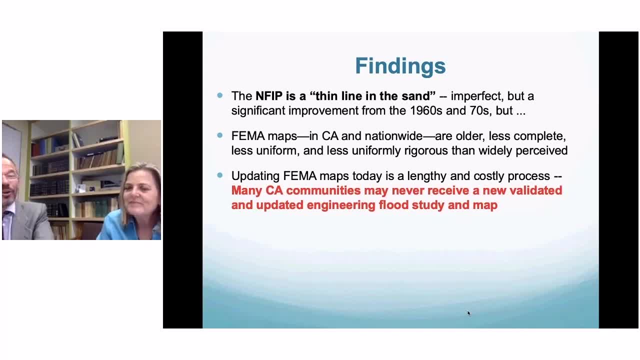 that was the state of technology when you were lucky during the earliest computerized flood studies leading to maps. So that the technology has improved. however, updating FEMA maps today remains a lengthy. actually it's become a lengthier and much more costly process, with the result as Kathy said. 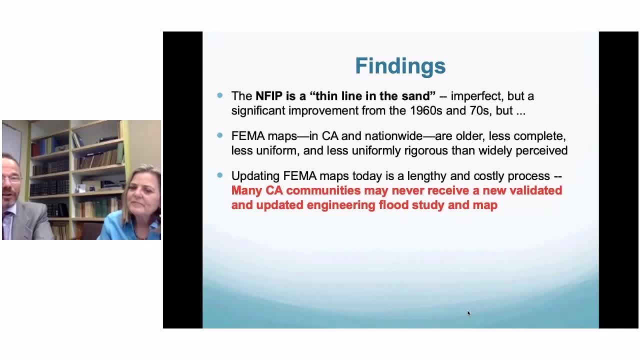 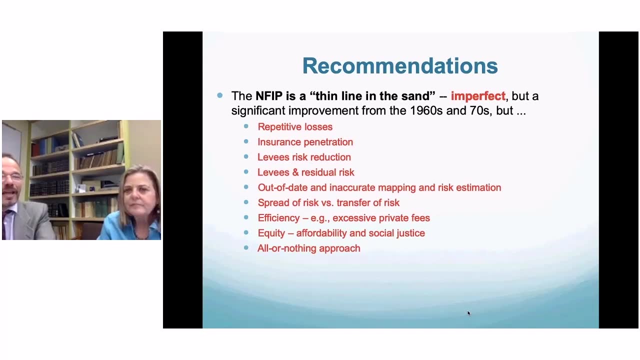 that many California communities today may never receive a new, validated and updated engineering flood study and corresponding flood map. So again, National Flood Insurance Program is faced with a number of different challenges, not least, currently, political climate in Washington. We have not talked much about reauthorization or reform. 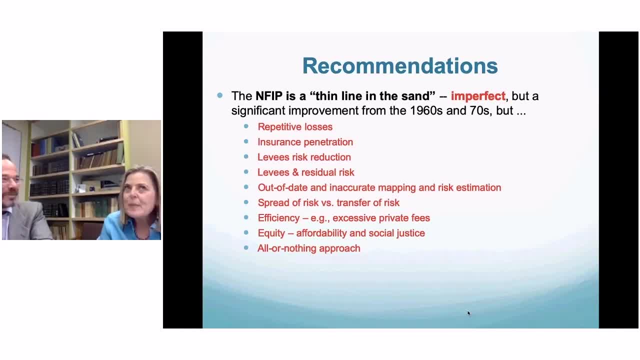 NFIP is current. We have not talked much about reauthorization or reform. We are currently on it. I think it's its 10th short-term extension. Yes, 10th, Something like that, plus or minus one. We lose count as these things come through with hopes for reform, but no promises and no success to date. 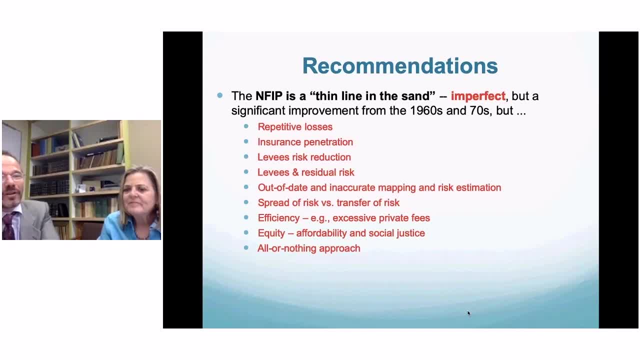 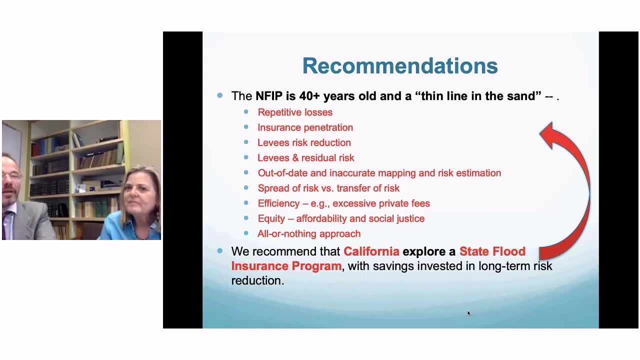 The suggestion by UC Davis, DWR and others is that California at least look at the possibility of a state-based flood insurance program. One of the potential benefits of that is that we have a wide variety of things that we can do together. benefits is to address some of the challenges facing NFIP on a nationwide. 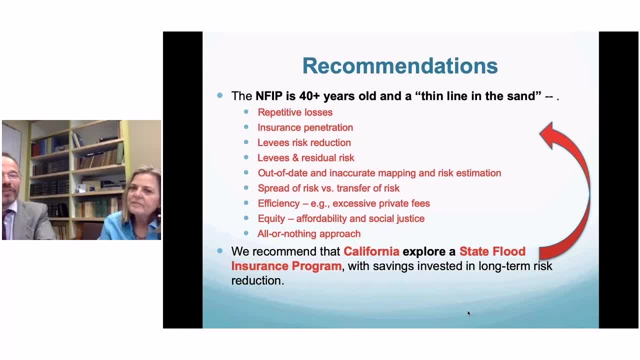 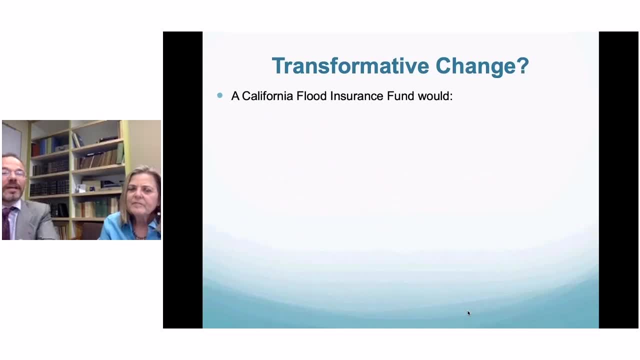 basis address those challenges, at least within the state of California and perhaps as an example for the rest of the country. Possible advantages of a California flood insurance fund. First for once, this is a potential revenue generator for the state, So this is not a big ask of additional investments. This. 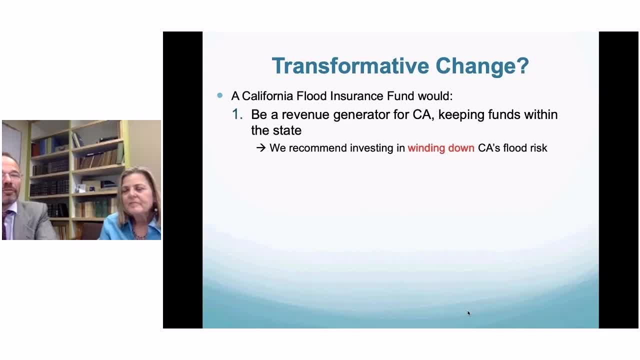 is a potential mechanism for keeping funding within the state, So particularly within the house. this is the the US Congressional House Reform Bill that was discussed. some of those profits, at least, would be diverted towards private insurers. So our suggestion is to put California's state into that game and 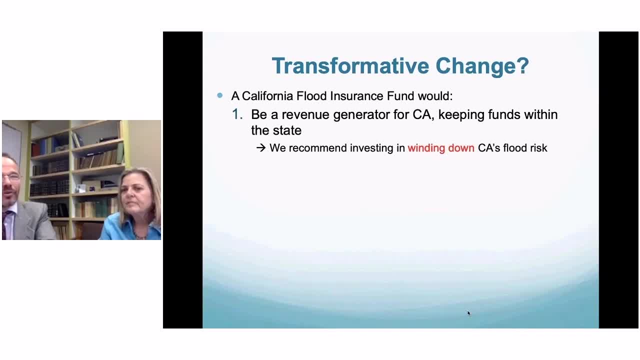 again, this is savings, at least theoretically, based on historical records on the neighborhood of two states. So we're looking at $200 million per year. Our strong recommendation is those savings be invested in winding down California's flood risk over time. This is also an opportunity for transformative change, both at the 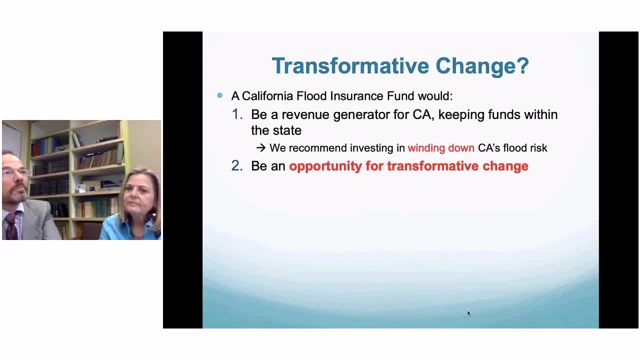 policy level, but also in how we conduct mapping and management of flood risk, again within the state of California and possibly beyond. So we suggest this is an opportunity to move from the current situation of flood hazard, which is essentially or widely understood as an all-or-nothing in or out of the flood zone, towards the future of flood mapping. 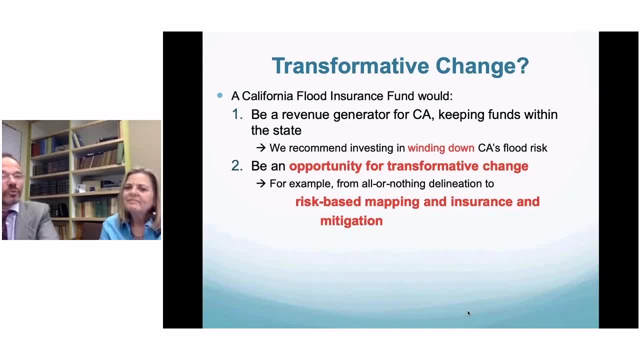 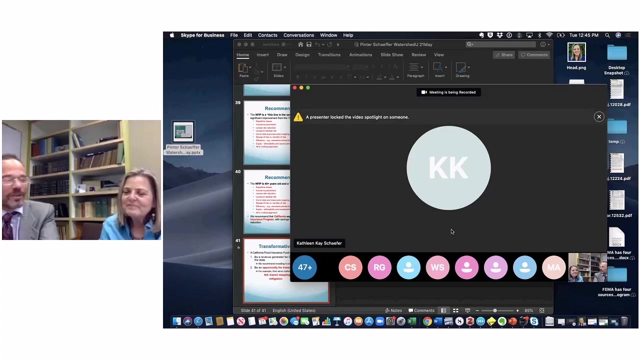 and this is happening elsewhere in the world and that is risk-based mapping and risk-based rate-setting insurance and risk prioritized mitigation within the state. So we look forward very much to discussion and thank everyone for their patience. So I can anticipate a couple of the questions. So we've been hit with a couple. 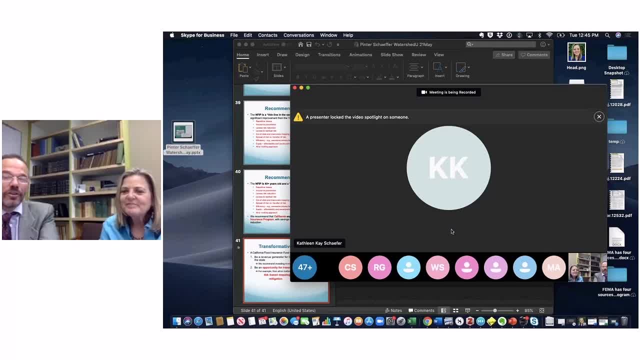 hard questions in these discussions, and so the first one is really out of what we mentioned: the big question of the analysis, So what Kathy calls the long tail risk, and that is the danger of another 18,. what was it? 51,, 52, storm and arc storm type scenario. The first real risk has been the high profile for the state, So that 18,, 51,, 18, 52 saw catastrophic flooding statewide across California and one could imagine if that opened again that California would not want to be on the hook for its own insurance risk. and 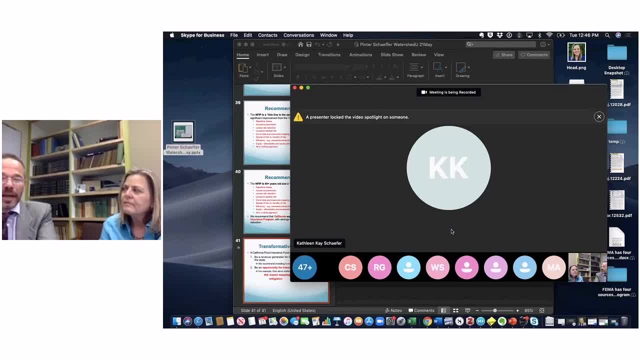 there's a lot of questions about that. how much of that risk has been mitigated through structural protections like dams and bypasses? I will defer to the engineers on that question, but what we point out is that the risk has been mitigated Wow. 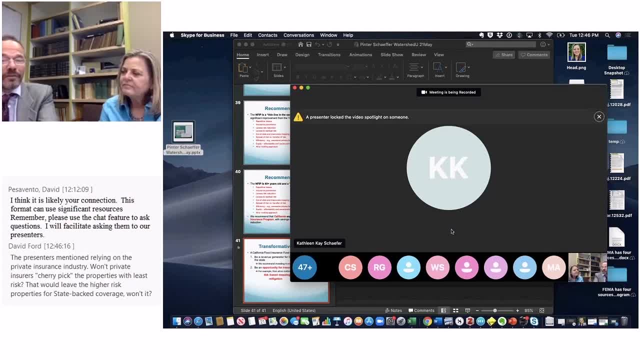 What we point out is, at least within the Central Valley of California, the state already owns that risk. That's right. So, following the precedence of the Paterno decision, California was held liable, within the state plan of flood control, for levee failures and ensuing damages. 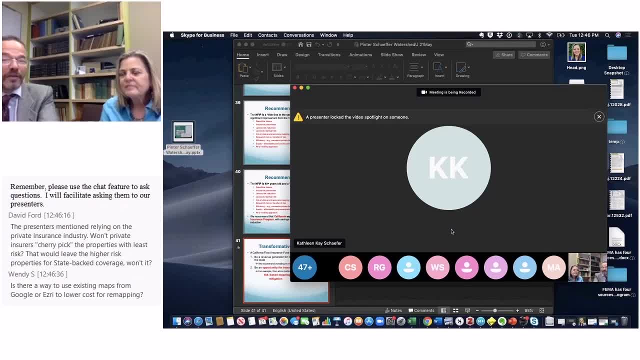 So we already own that risk, have paid. I've heard numbers in excess of a billion dollars when legal fees were factored in. So the proposal here is, if we already own that risk, might as well insure it as a way of essentially mitigating it. 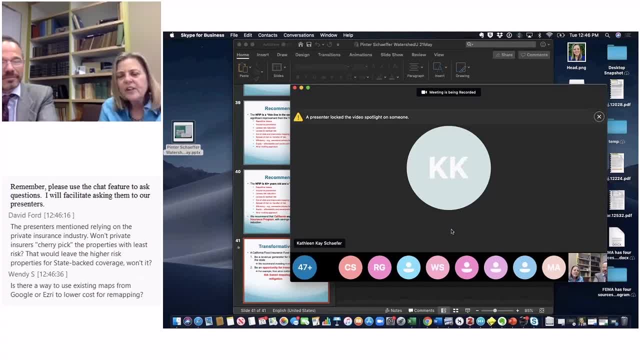 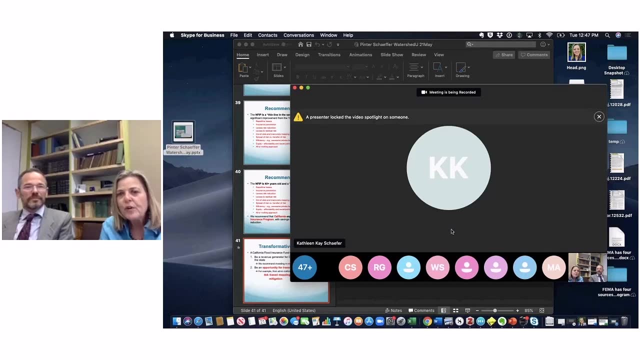 And then, I would add, I have done some work on a study that I hope to publish later this year, where I examined the payouts from the National Flood Insurance Program and from the Disaster Assistance Program, from the Public Assistance Program and the Individual Assistance Program. 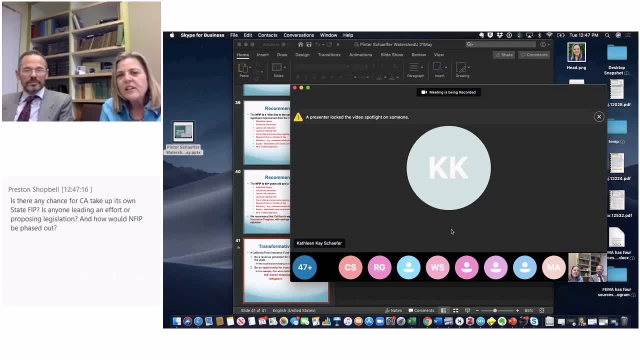 And what I found was that the combination of the three- the individual assistance, the public assistance and the NFIP- still are greatly lacking in providing enough money for communities to really recover. So if we did have a catastrophic loss, we would be completely uninsured or underinsured. 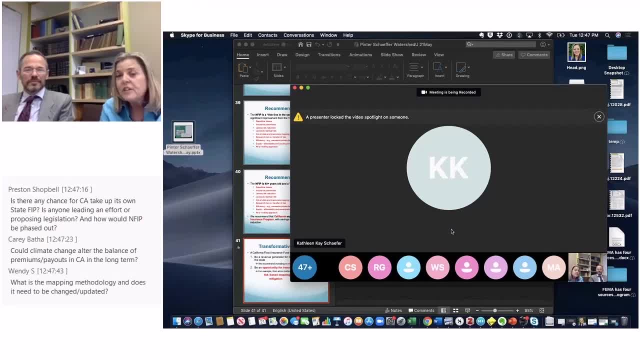 and finan. It could Financially be very devastating for California. So an alternative would be, or could be, to examine some sort of catastrophic flood insurance bond that would cover us for those rare but very damaging and very consequential floods. Great, thank you. 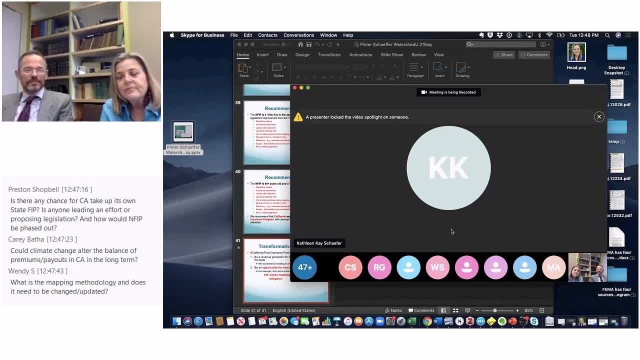 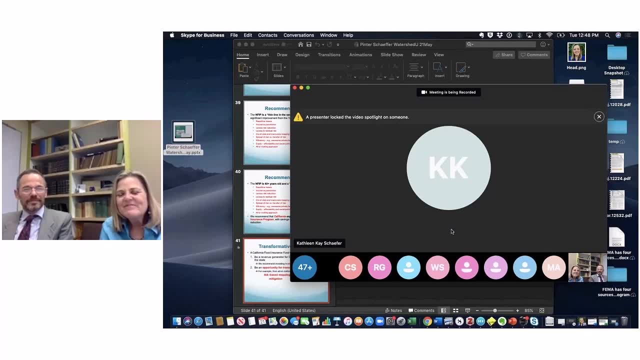 We do have a bunch of questions that are coming in now. Let me start with one I got on e-mail Question about the research. Did they find any information on how many new structures are being added to existing known SFHAs? That's a great question. 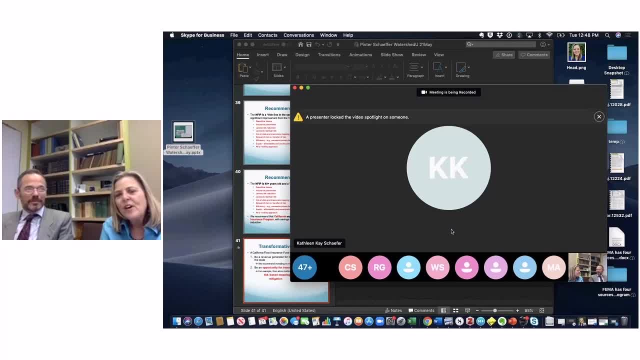 That's one we haven't had a chance to delve into, but one that I'm interested in. I've looked a bit, tried to look a bit- at the Plan Bay area and the consequences of the plan Bay area, Because in the Bay area there is a desire to have walkable, livable communities. 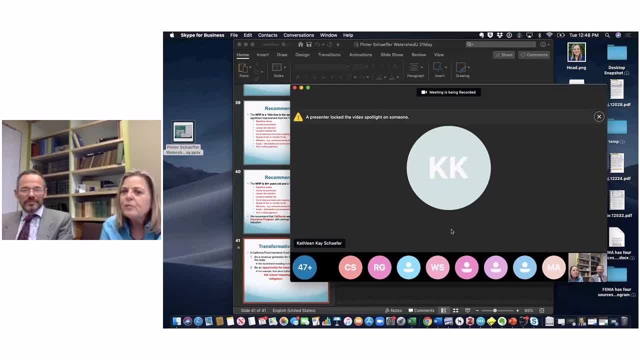 And you have to ask where is the best location for walkable, livable communities? It's in areas that are flat. Where are areas that are flat Next to the Bay? So there's a question I have about that. But yeah, that's an area of research I'd love to explore. 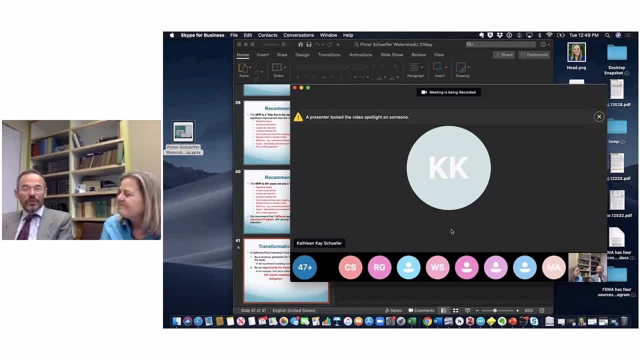 And there are hints that there's some of that going on In the worst case are Yeah. So again, the analysis of the repetitive loss structures in California is again this is ongoing, but it shows a number of not just flooded properties but repetitively. 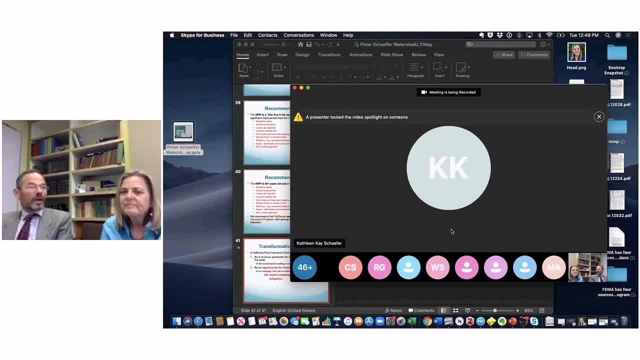 lost flooded properties within the 100-year flood zone. So it's within and without, And really what worries me is structures that are just outside the line. So, given climate change, intensification of flooding Again, what is a legal structure to be built today could be if the maps were ever updated. 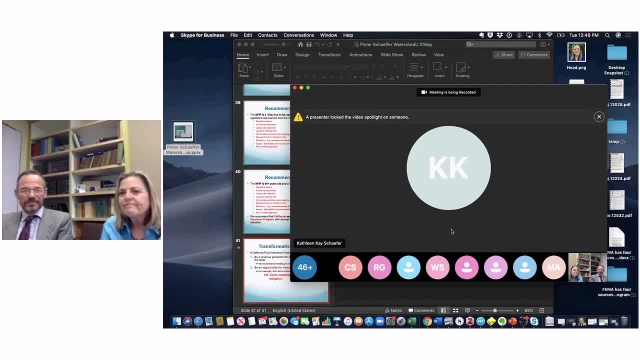 within the hazard zone in the future? Great. Another question: Could we adjust the NFIP to require that the state or perhaps local governments pursue mapping in order to be eligible for NFIP coverage, and maybe on a 10-year basis? Has that idea been? 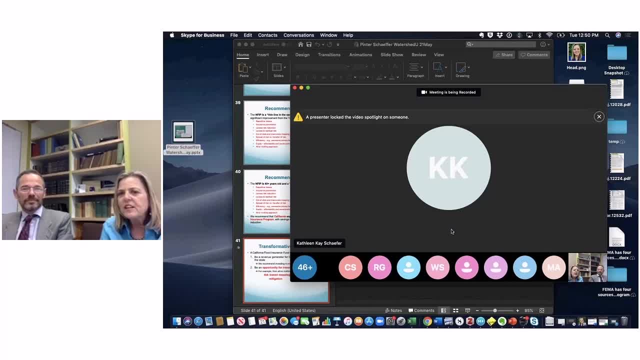 Yeah, That's one of the items that's listed. One of the items that's listed in the current proposals. Maxine Waters is currently the chairman of the House Finance Committee, where the bills for whatever happens will originate, And having a community-led mapping effort is listed in one of the bills. 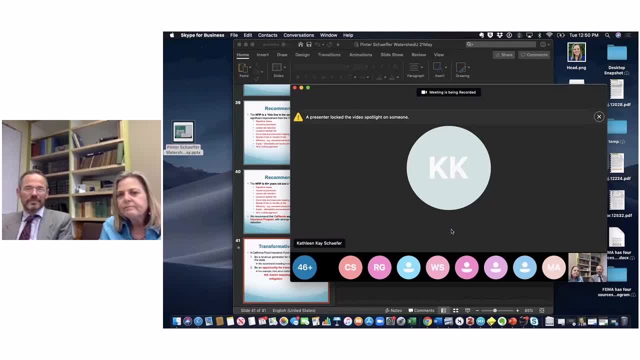 Great. Another question, A bunch of questions from the chat. First one: Will private insurers be relying on private insurance industry? Won't private insurers cherry pick the properties with the least risk? that would leave the higher risk properties for the state back to coverage. 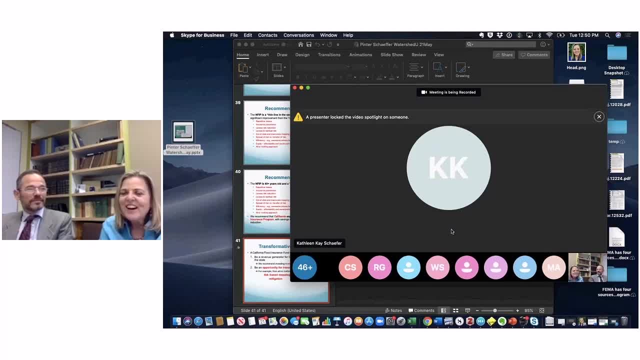 Won't it? That's a very common question And while I'm not an insurance expert, I do sit on some monthly calls from the private insurance sector And I will tell you that the private insurance sector is very interested in moving into the market. 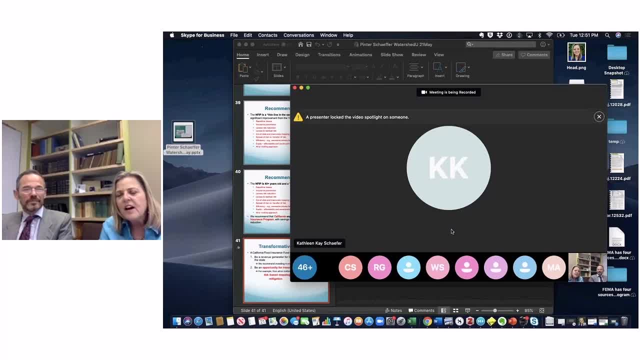 And the study recently conducted by Milliken found in Florida, for example, that virtually the northern half of Florida overpays in flood insurance And the southern half of Florida underpays. So you could see where the private sector would greatly move into the northern part of Florida. 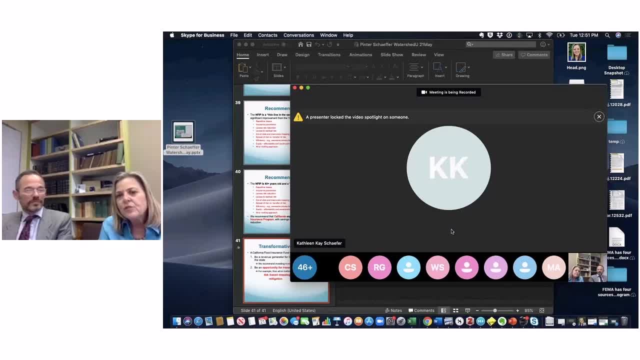 And again, may not insure as many in southern Florida. But the other part of it is that we are so underinsured that you could make the case that with the advent of public or private insurance will fill that insurance gap that's been missing. 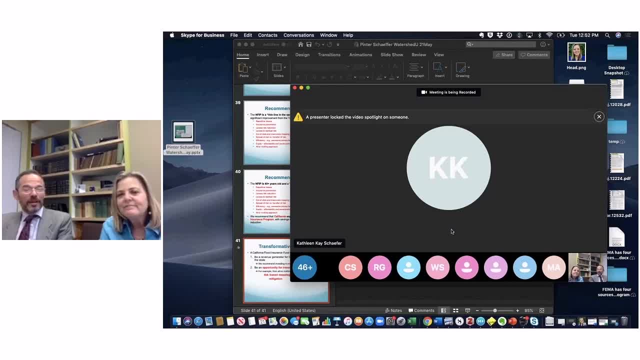 So that's a positive spin on it. The negative, I would emphasize, yes, I think My opinion is, the private insurance industry will cherry pick, And so I would suggest, just personally, that's a motivation for California to stake out this territory while the opportunity exists. 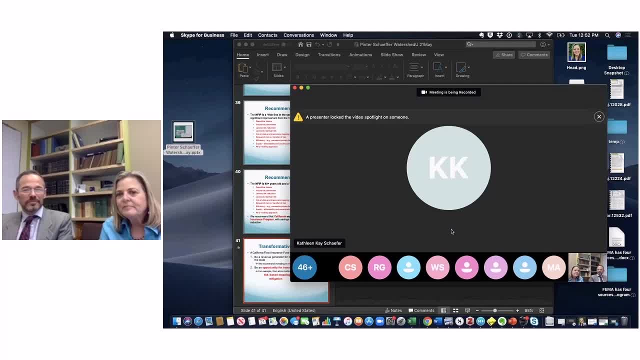 Great, Thank you. Next question: Is there a way to use existing maps from Google or Esri to lower the cost for remapping The Google and those maps aren't really the best tools. There are a number of companies moving in. There are a number of companies moving into the catastrophic modeling arena. 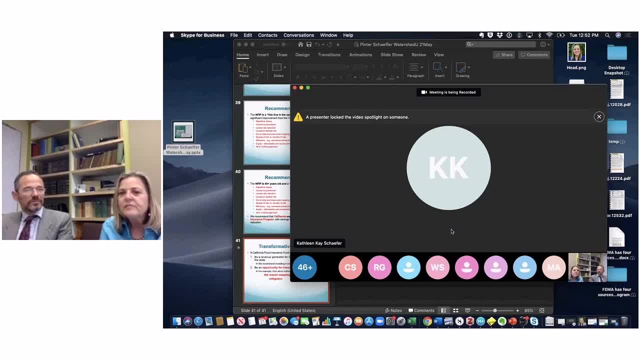 And there's a real movement to do so. We've got a Twitter feed from RMS, which is one of the leaders in catastrophe modeling, that I believe in 2020 they plan to make their models open source, which is very exciting. So I think that's an area that you'll see a lot of movement and a lot of exciting transformation. 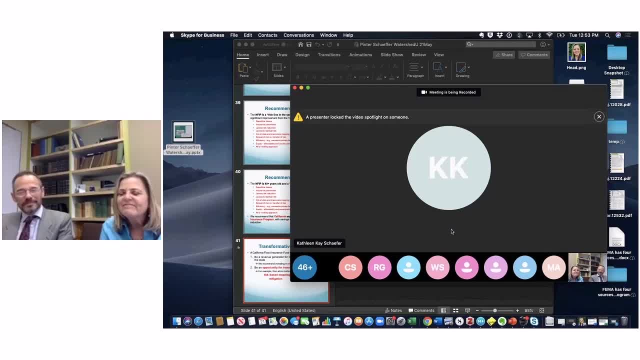 So not Google Earth yet, but there are other alternatives. Yeah, Thank you. Has there been any discussion with the feds about splitting their program? Would this impact home loans? since home loans are nationally backed, California would need federal support to take on this program, which seems unlikely since we're helping to pay for other parts of the country. 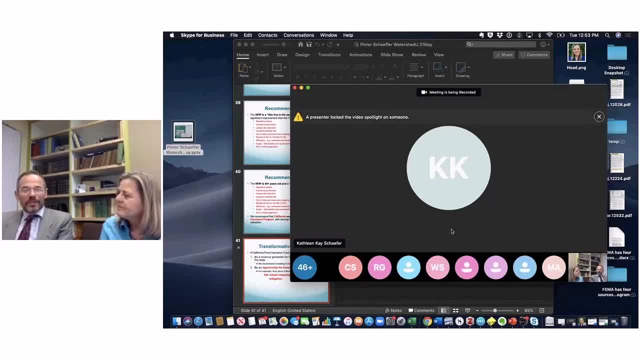 So we need to clarify that no part of this proposal involves an exit from the national flood insurance program. That is federal law, That is the law of the land. NFIP, underwritten flood insurance, Flood insurance or flood insurance of some kind is a requirement for federally backed mortgages on a nationwide basis and that is not anticipated to change. 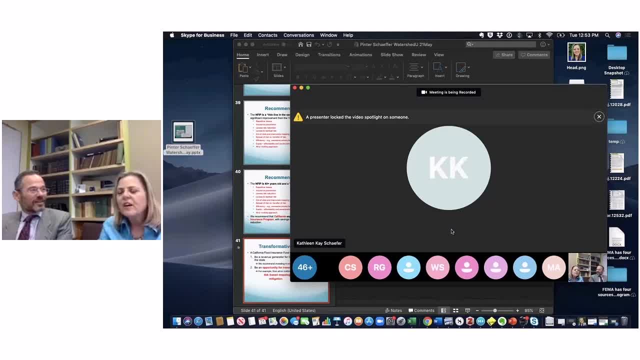 But a little clarification. So the communities must belong to the national flood insurance program in order to be eligible for all kinds of disaster assistance, whether it's hurricanes or earthquake. However, what we're talking about is alternative to the FEMA standard policy or the NFIP standard policy. 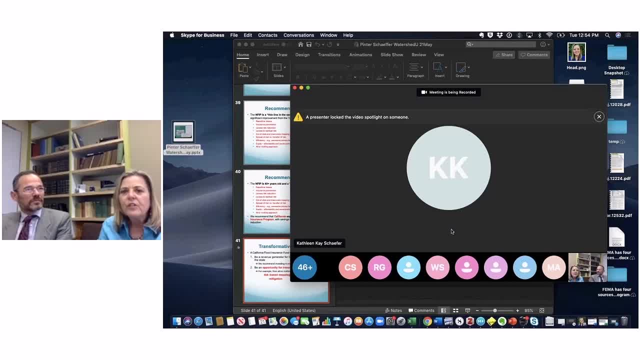 And there is a new law that has been put in place that allows for or supports private flood insurance under certain conditions, And we would just be following that law. There wouldn't be a significant difference, Just adding a state-based alternative to what is already moving towards a variety of options, including private insurers fulfilling the NFIP mandate. 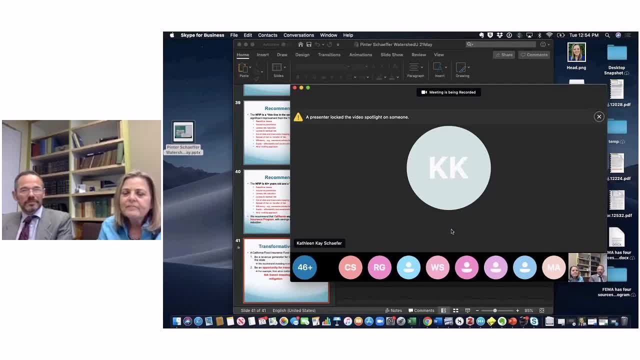 Thank you very much, And that kind of goes into this next question. Maybe you can just briefly comment on it. Is there any chance for California to take up its own state flood insurance program? Is anyone leading an effort or proposing legislation, And how would NFIP be phased out? 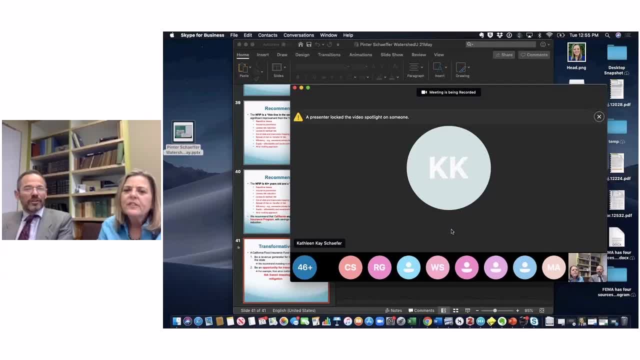 So I think that kind of overlaps, but maybe you can chime in a little bit. So again to clarify, NFIP would not be phased out. California would be exploring- and that's all California is doing now- its options under existing NFIP authorization. 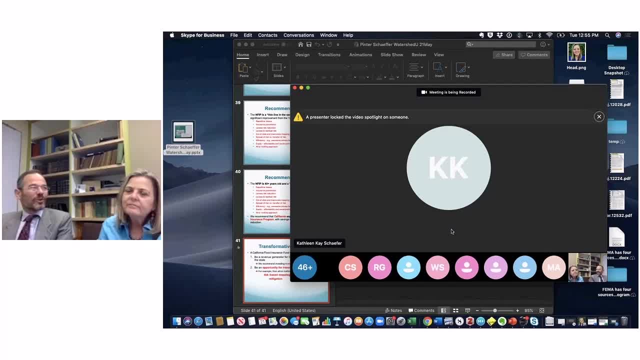 And there's interest in this. No one is writing legislation right now. Part of our goal here today is to help move that discussion along. That's right, And, in addition, one of the bills that we're going to be talking about today is a bill that we're going to be talking about in the next few weeks. 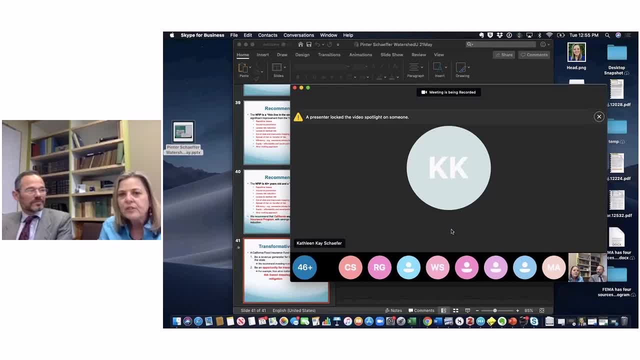 One of the bills, one of the House bills that Maxine Waters has before her does have language directing FEMA to examine the opportunities for a community-based flood insurance program. Previous iterations of the bill encouraged FEMA to consider- excuse me, consider- a community-based flood insurance program. 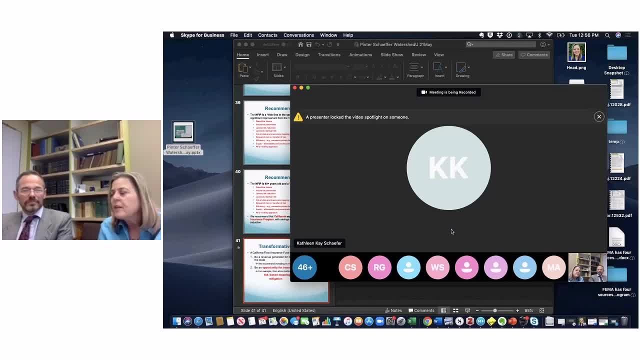 But the new legislation actually now makes that mandatory That if those laws go into effect, those bills are passed with the reauthorization, then FEMA would be directed to study as a template, a community-based, and we would encourage or want or ask that California have one of the communities that's under consideration. 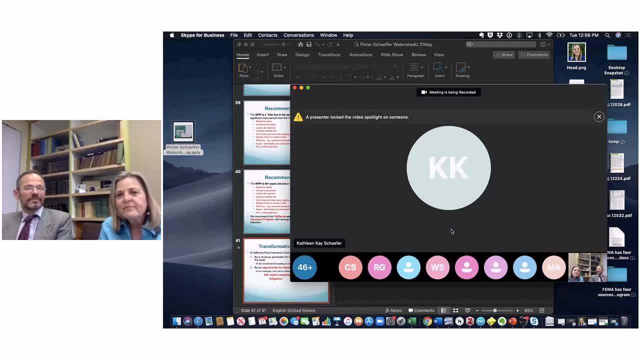 Excellent. So I have two more questions. One is: could climate change alter the balance of premiums? slash payouts in California in the long term? Yes, So one of the potential solutions or benefits of California is that it could do what the feds currently are unable to do, and that is examine non-stationary hydrology, including climate change. 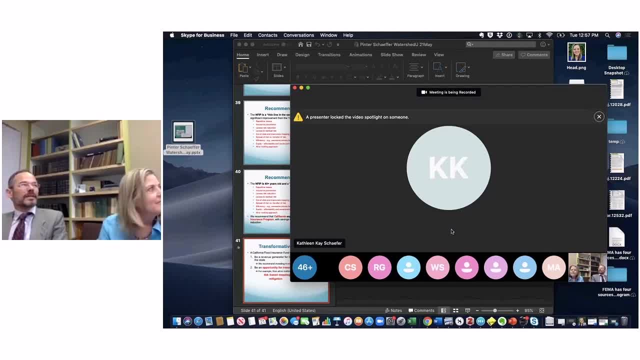 I was just asking if we have four minutes to an oral exam. Yes, thank you, Thank you. Thank you. Thanks for being part of the university. Welcome to the university, Yep, no problem. And then the last question: what is the mapping methodology and does it need to be changed or updated?